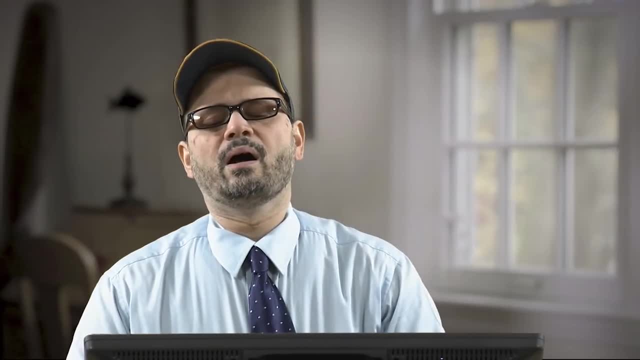 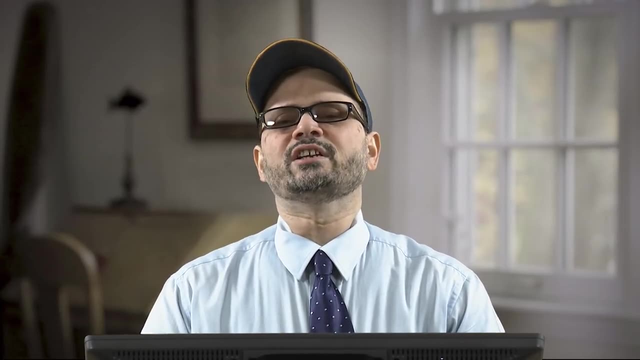 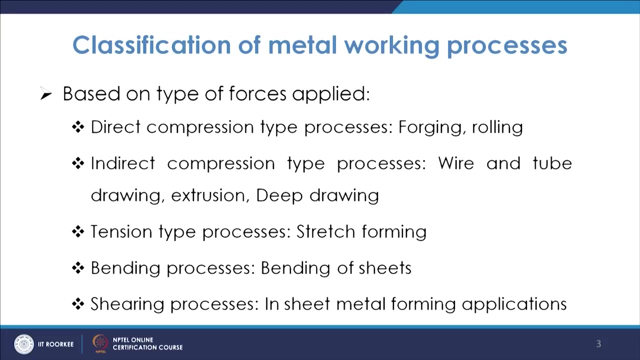 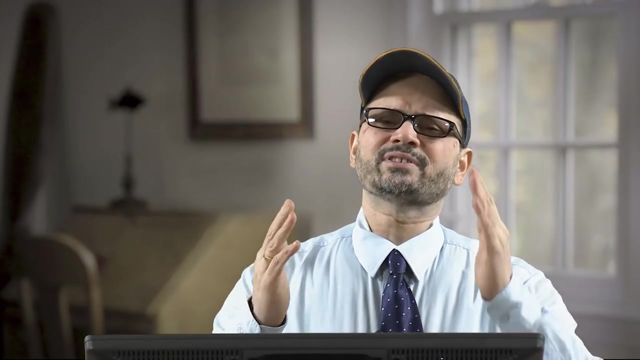 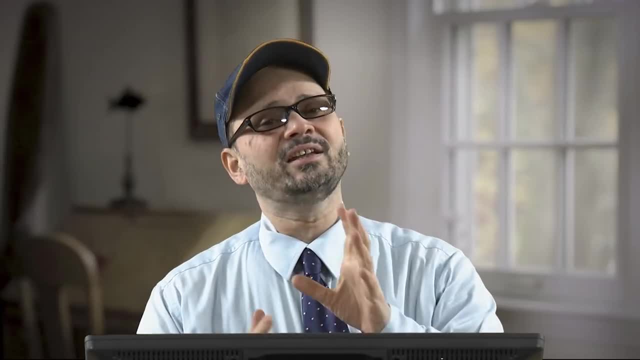 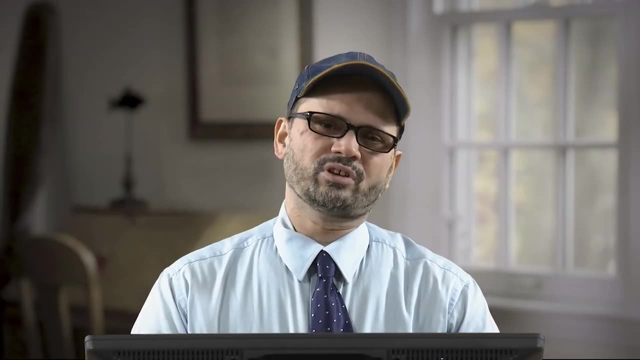 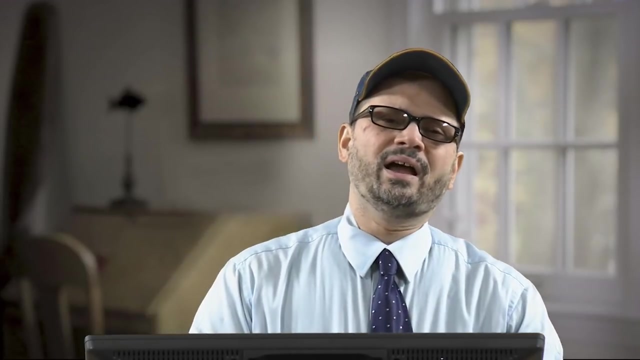 Indirectly applying the compressive force. we are indirectly. basically the compressive force is applied and that basically creates the deformation and it is. example is wire drawing or tube drawing. So as you know that in wire drawing you are pulling And then at 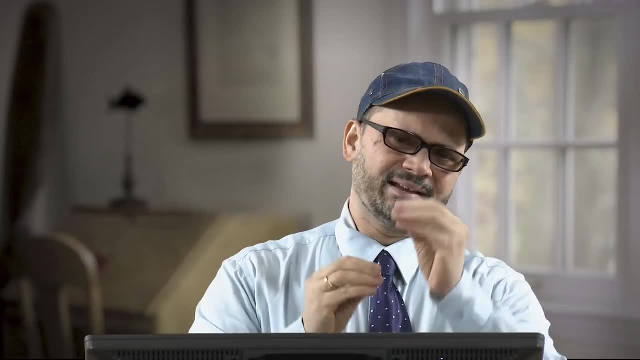 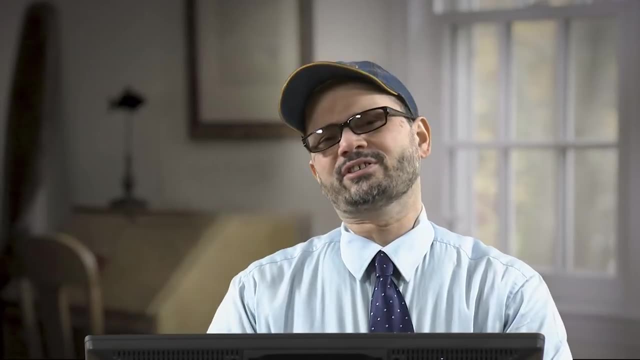 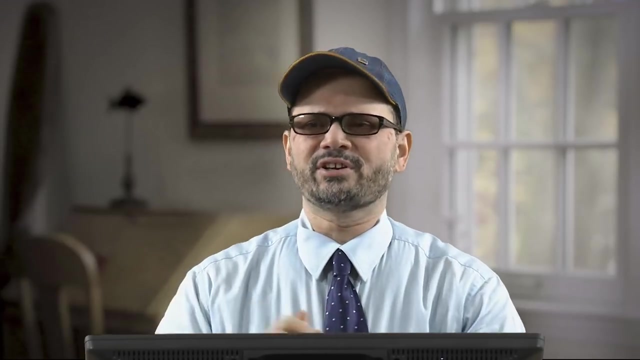 the die exit, you know. and there, when, where the bar or the billet which is in contact at point, the compressive stresses are developed, compressive forces are developed, And because of that the local failure takes place and then the material comes out. So that is your. 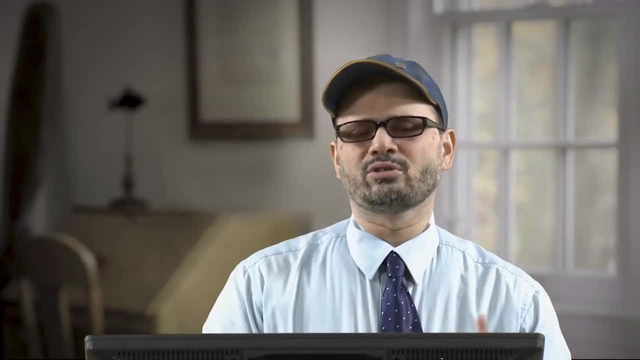 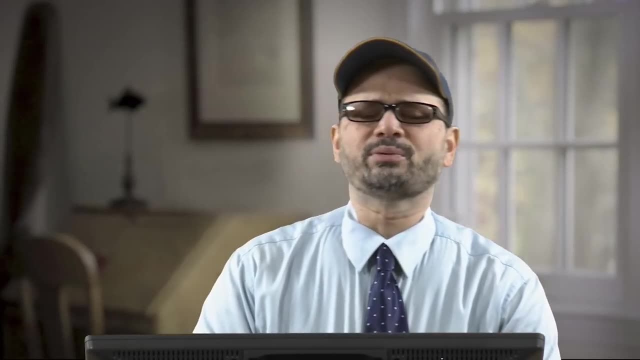 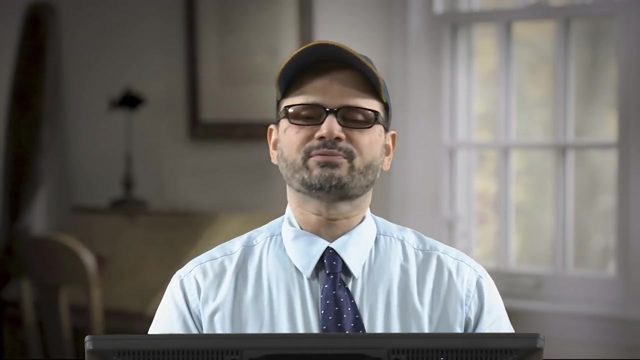 indirect compression type, similarly tube drawing, extrusion, also the same thing, and deep drawing. So we will discuss about them. The tension type processes where normally, because of the tension force, this deformation takes place. an example is stress forming, where you have a form block and you are applying. 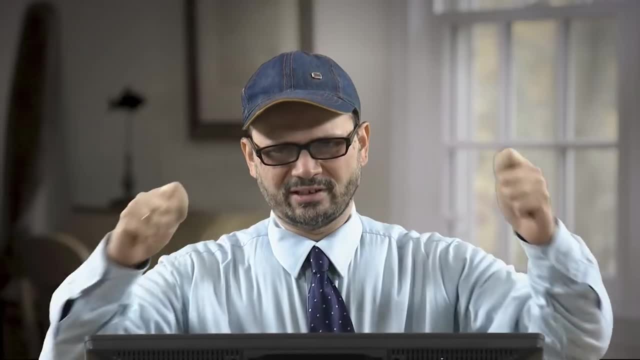 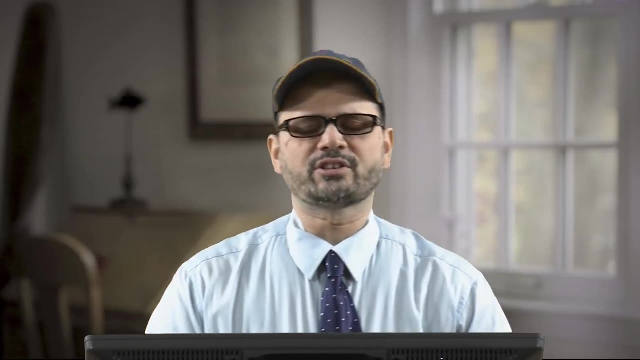 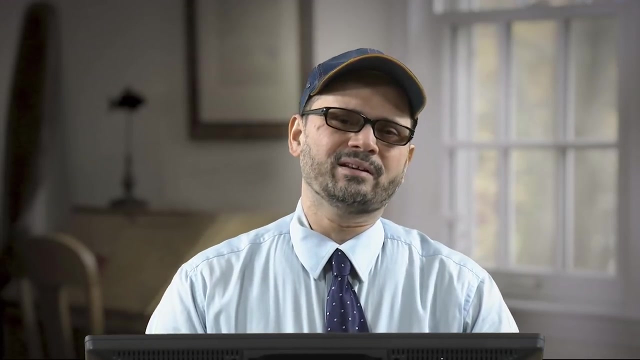 you are, you are stretching a sheet in that case. So it will, due to the tensile stresses developed, that deformation takes place. So that is stress forming Bending processes, where we apply the bending moment to bend the specimen and in that case, the material. 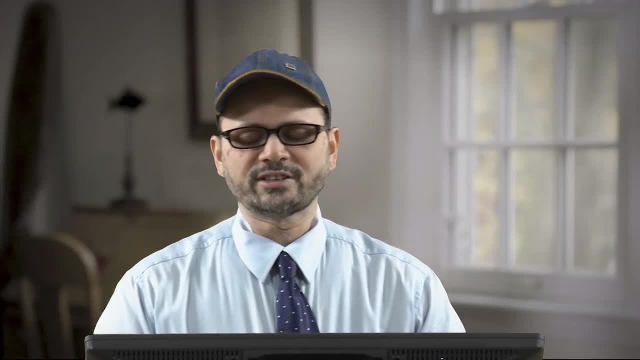 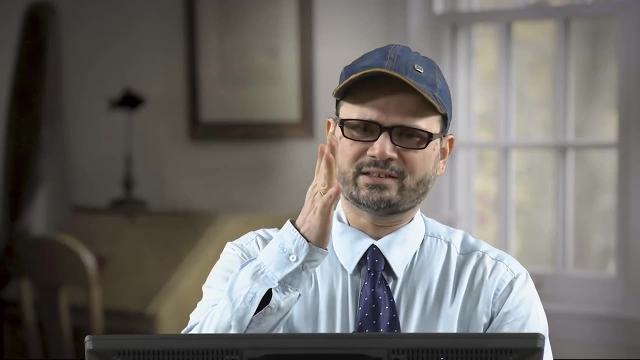 bends. So that is bending process. Similarly, shearing process And shearing process. you have blades, So you will have the from the top and bottom. you have two blades and they will be shearing, cutting. So because of that, the failure takes. 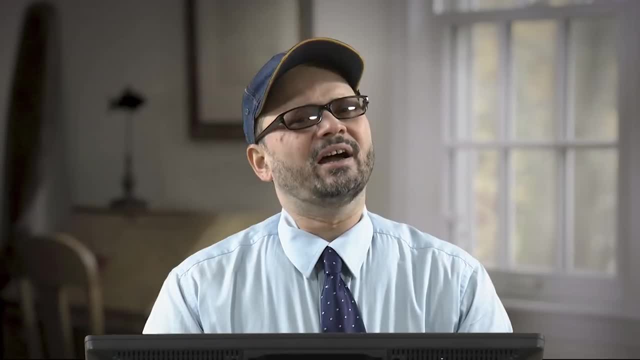 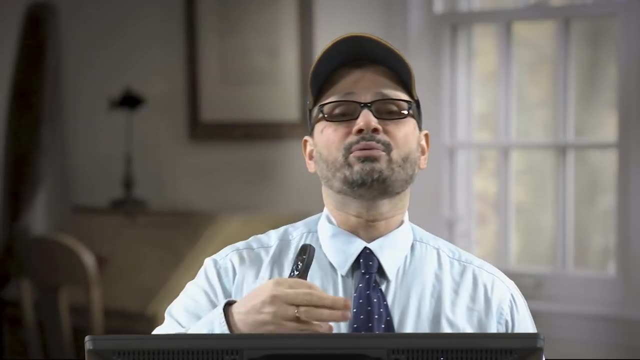 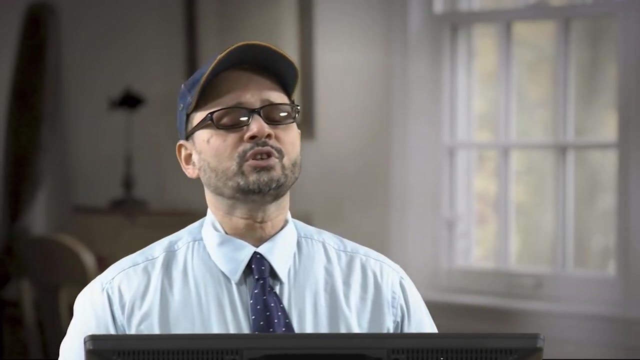 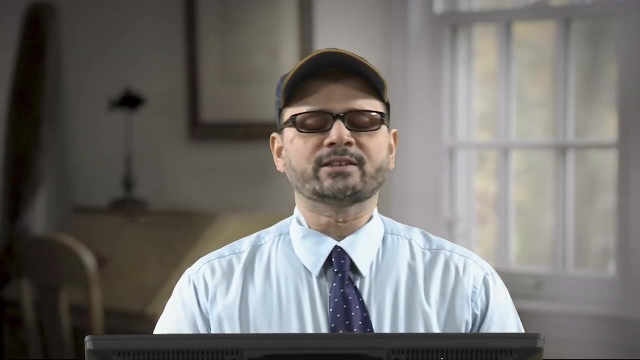 place and then the deformation takes place, So that these are basically the different types of forces because of which the deformation takes place, and we will talk about them one by one. So first is the deformation. So the deformation is the direct compression type forces. Now in this the force is applied to surface of 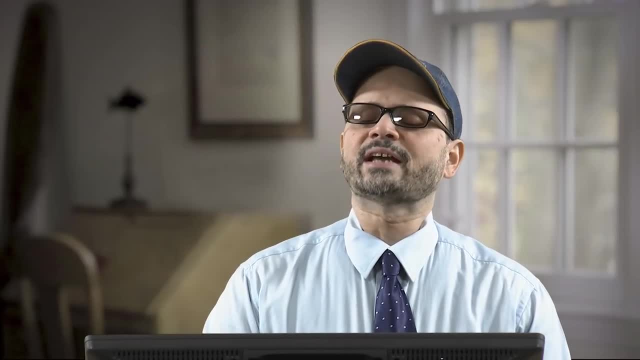 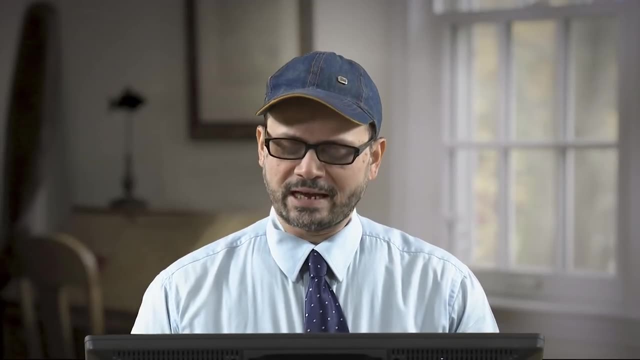 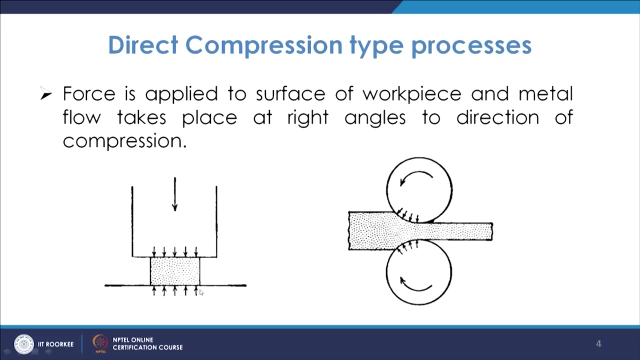 work piece and an and metal flow takes place at right angles to the direction of compression. So in this case, the example is as we discussed: it is forging and rolling. So if you see, this is forging and this is the rolling. Now, in this case, as you see, in forging, this is 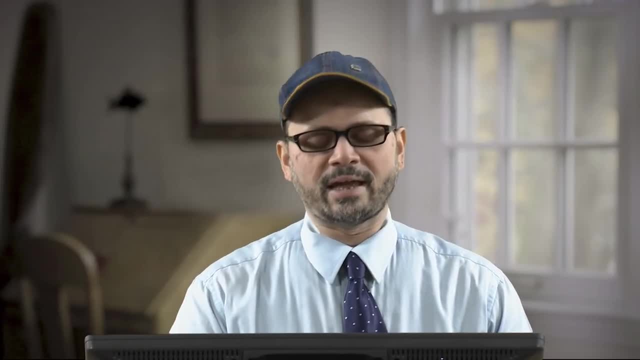 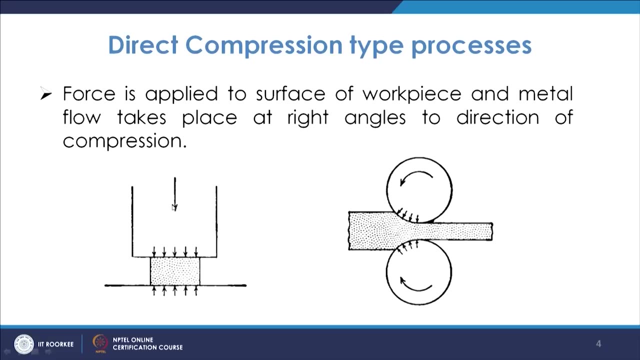 the top die, and this is the bottom die. So you apply the pressure. from here you are, apply the compressive force, as you see, and this job is subjected to the compressive load, and then, because of the compressive load, the material deforms and it goes. So you are. 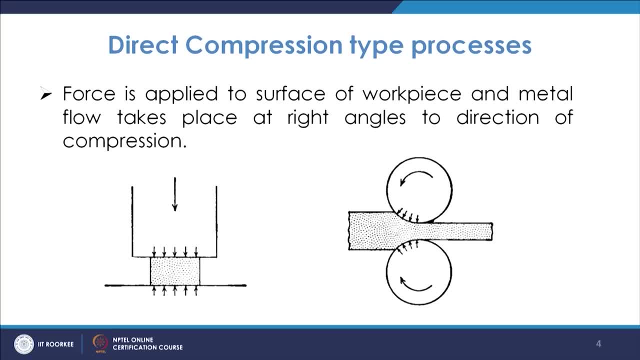 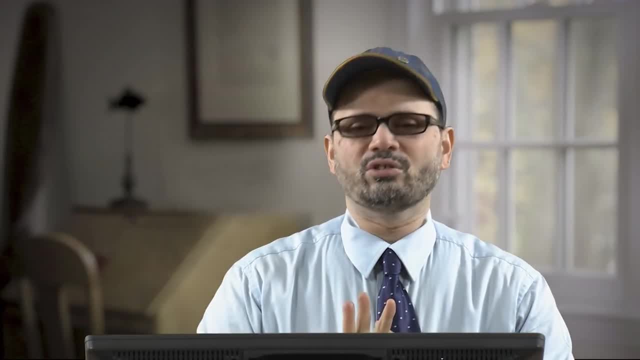 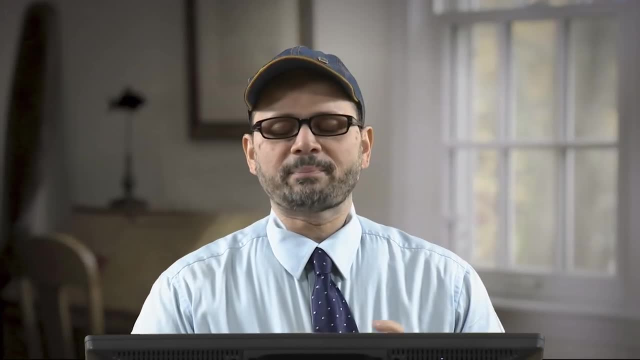 applying the- you know- force in the vertical direction. So in the vertical direction or z direction, and the material? if you are keeping one of the dimension constant from both the sides, then the material will flow in x direction. So this way the flow will take place perpendicular to the direction of the applied compressive. 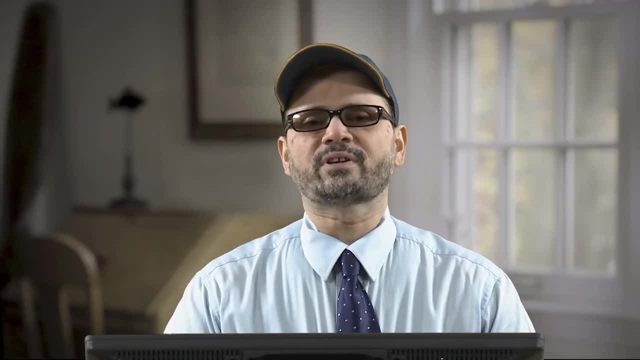 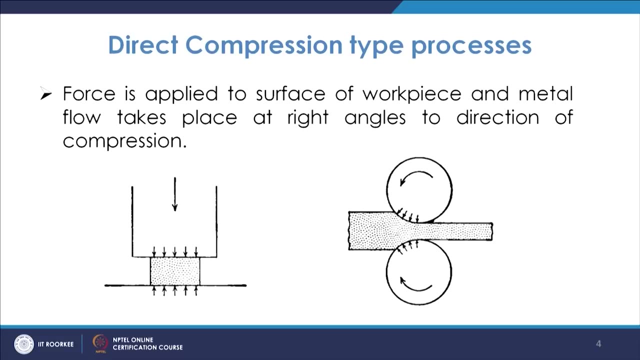 force. So this is the normally case in the case of direct compression type process. So, coming to the direct compression type processes, So we discussed that we apply the force to the surface of the work piece and metal flow takes place at right angles to the direction of compression. So the example is forging. 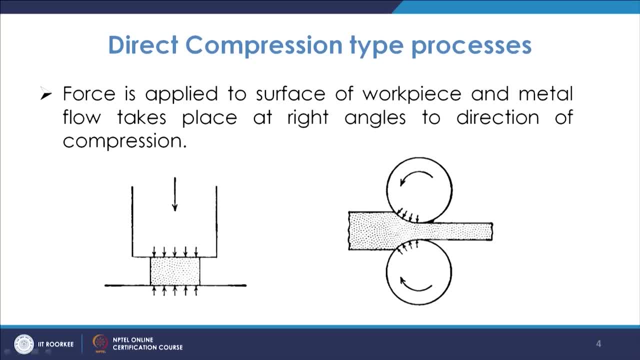 and rolling. So what we see, this is this is the forging process, and this is the forging process and this is the rolling process. So what we see is that in this process, in this forging process, this is the top die and this is bottom die, and the work piece is kept in between, and So this will be your work. 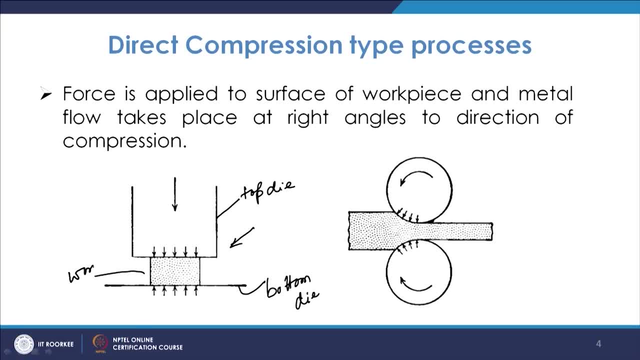 piece. So this is your work piece. Now, the further thing is that it will be expanding either in the x direction or the y direction. If it is the z direction, in that case it will be changing in x or in the y direction. So that way, basically, you are. 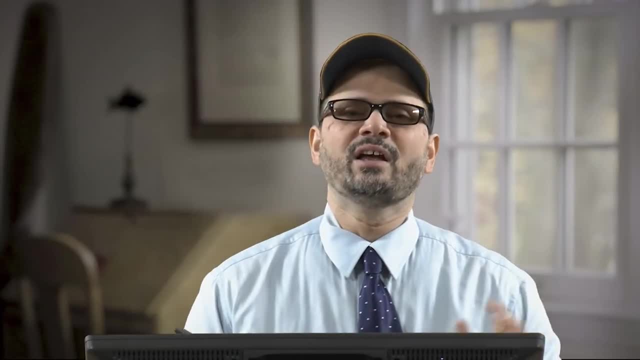 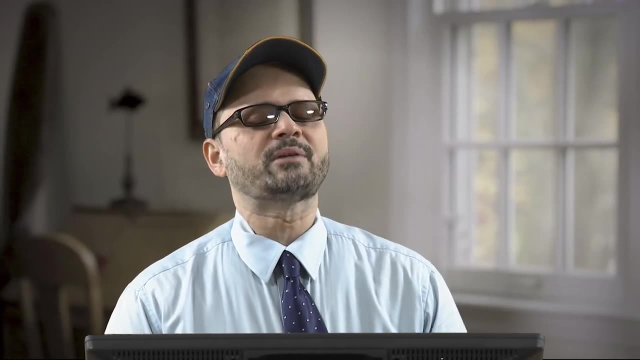 applying the compressive force in the z direction and it is able to flow in x or y direction, which is perpendicular to z direction. So this is because of the direct compression type of forces and this deformation takes place here. Similarly, direct compression type force is: 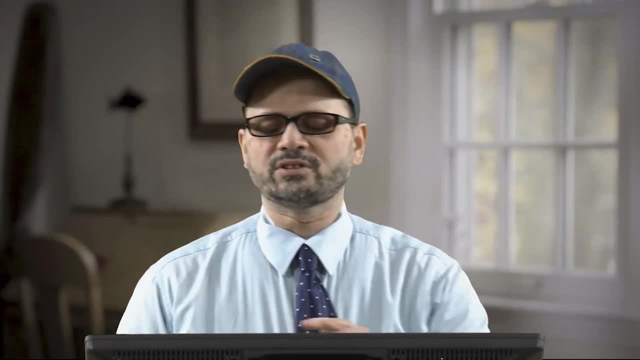 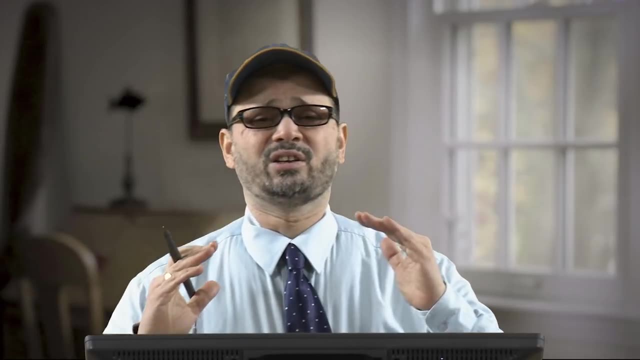 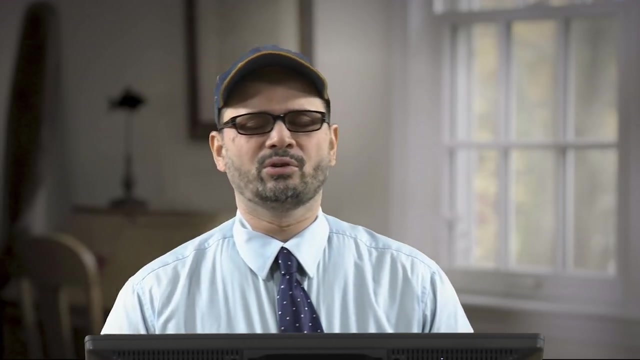 also applied in the case of rolling. So in the this, this rolling process is very common. in the case of industries where you are trying to decrease the cross section of the larger you know products like you have ingots or blooms or so, So in that case you are passing. 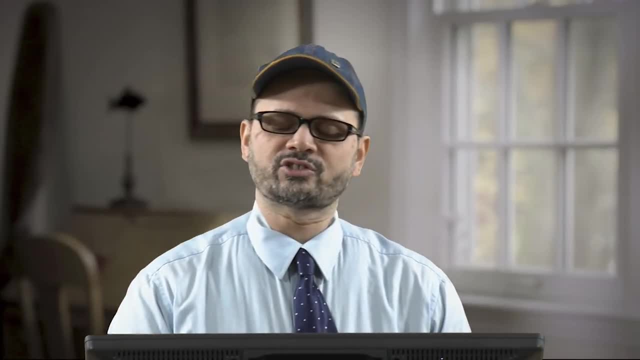 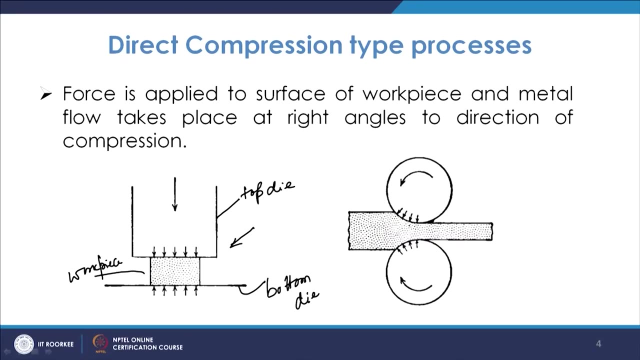 it through the two rolls. So the rolls are extremely hard and they will be rotating in the opposite direction. So what happens? when they come in contact with this, this, this job, then they are applying the compressive stress and in that, the material. 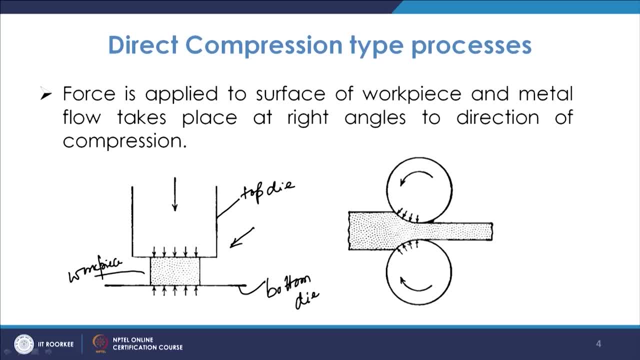 will be compressed and then they try to flow through the exit. So if you look at the compression here, so it will be compression in the vertical direction and then material flows in the, you know, horizontal direction. So basically these are the examples of the direct compression type of forces and the 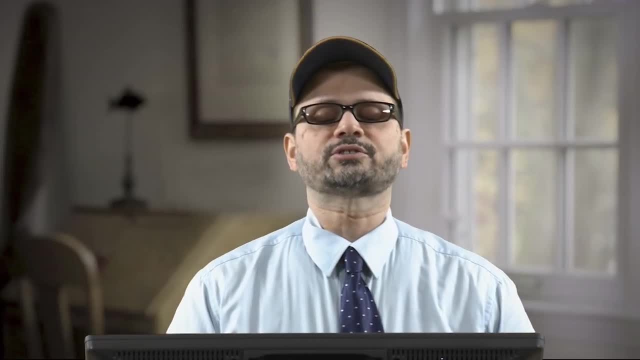 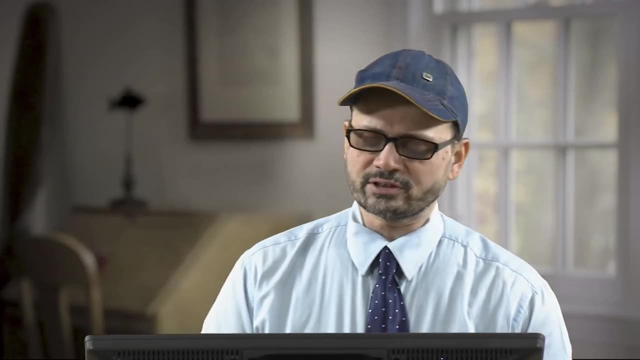 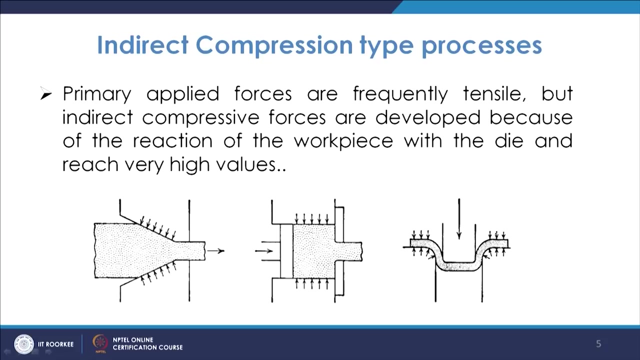 forging and rolling is the example of such process. Then you have indirect compression type forces. Now, in the case of indirect compression type forces, normally you primarily apply the forces which are tensile but then indirect compressive. So these two forces are developed because of the reaction of the work piece with the 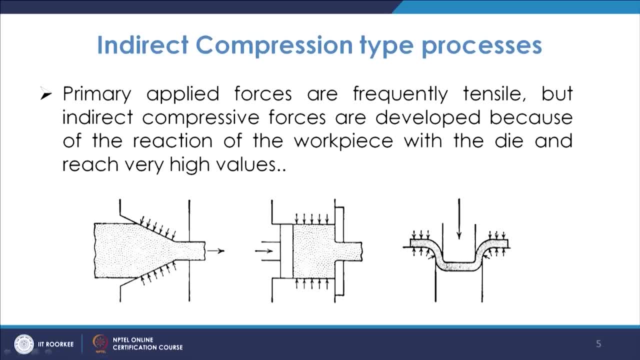 die and they reach very, very high value. Now, what is happens in these cases like this is your tube drawing. I mean, this is a wire drawing. So in the case of wire drawing, what we see is you apply the force in this direction, you are basically pulling. So you are primarily 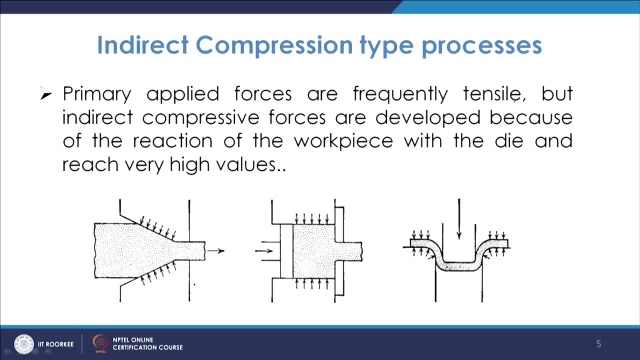 you are taking the tensile type of primary primarily you are applying the force. but but then what happens? this is the die. So this material billet or so, now it is in touch here. So once you pull here from here, once they are in touch, there will be reaction forces. 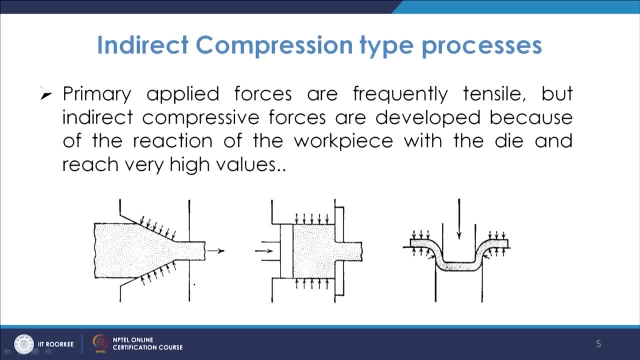 generated Now: the reaction force which is generated at the work piece and the die interface here. So, because of the basically what happens, that force is normally compressive in nature. 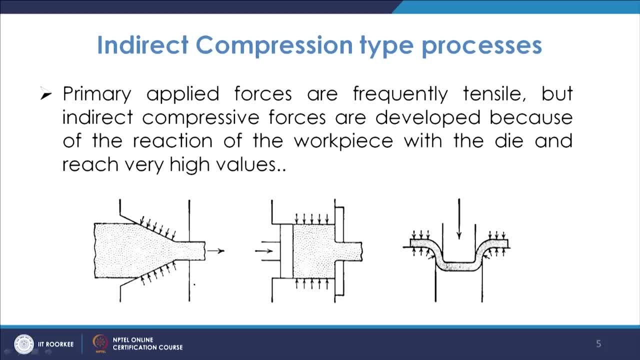 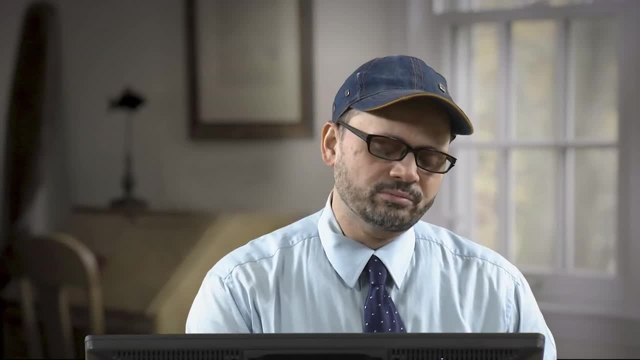 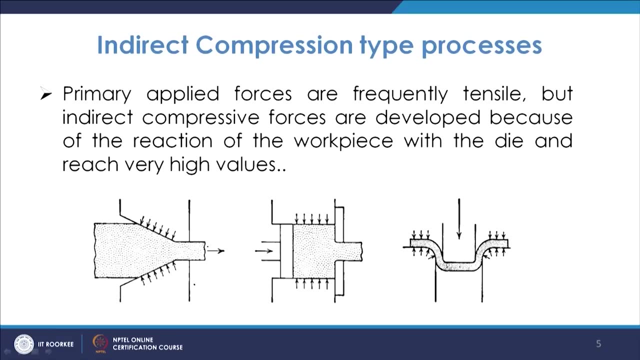 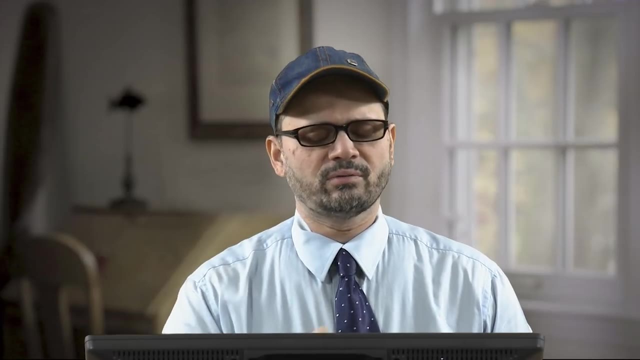 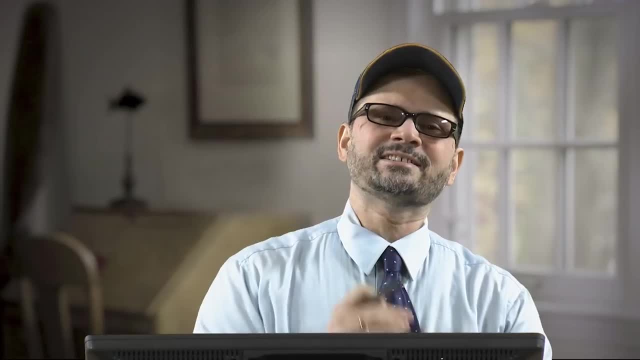 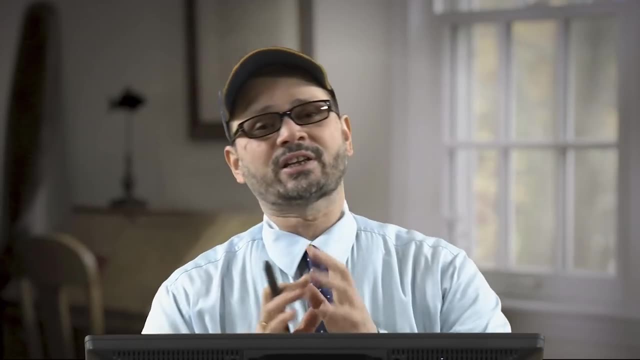 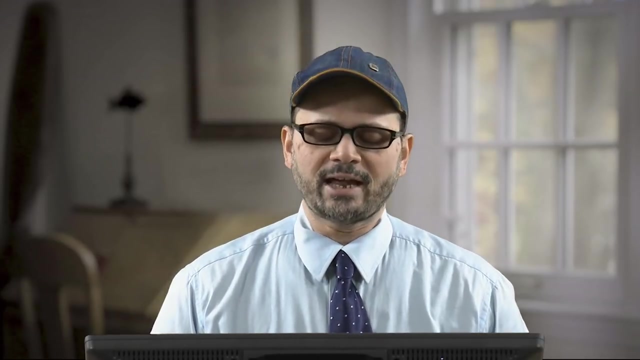 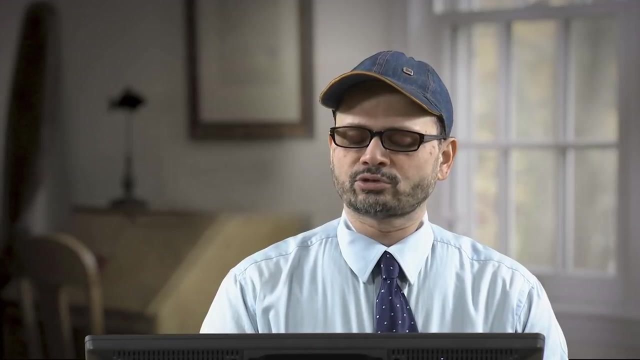 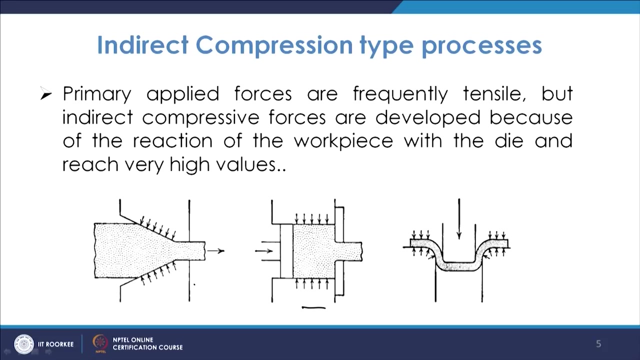 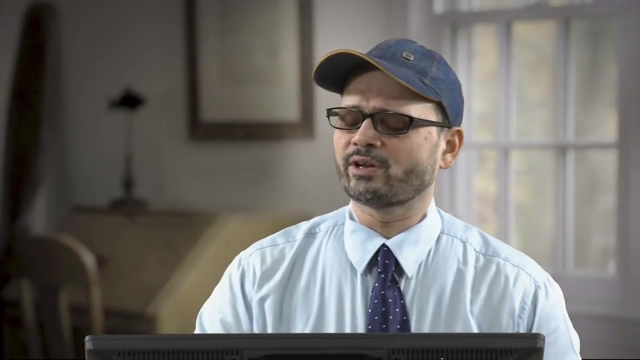 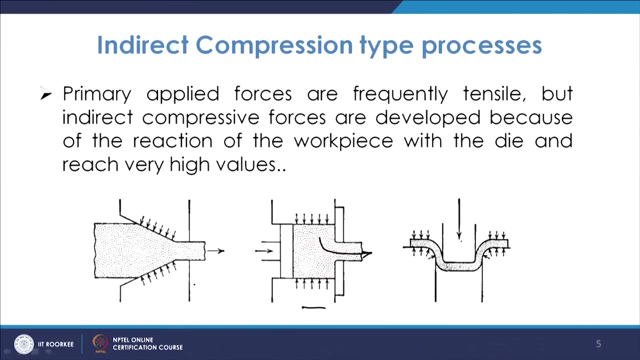 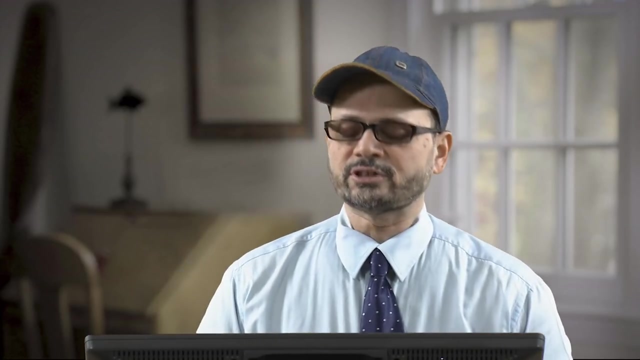 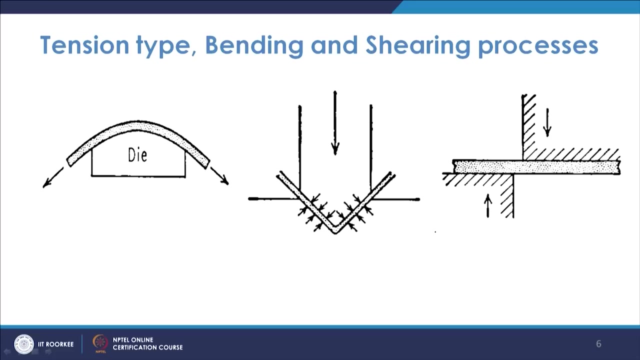 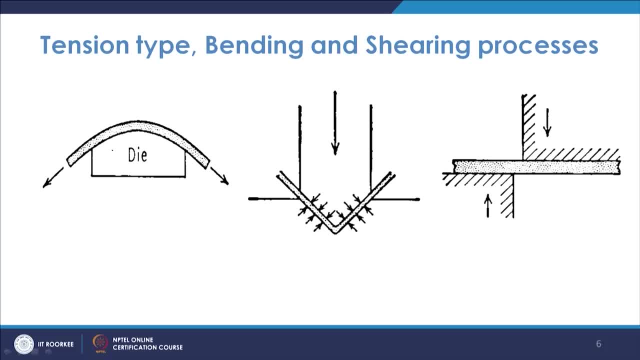 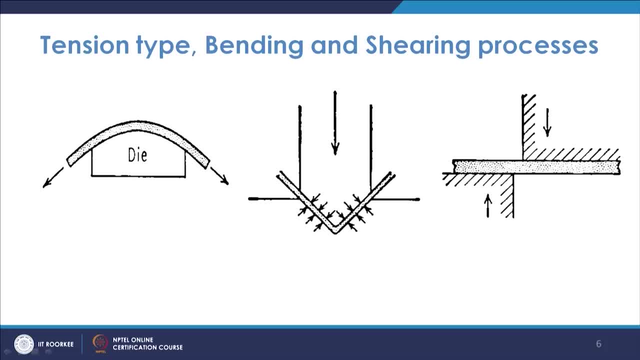 Similarly, you have the shearing process, where you have these blades, so top and bottom, and then once they will move in the bottom and reaction will be there at the top. So at this point there will be a shearing taking place and cutting 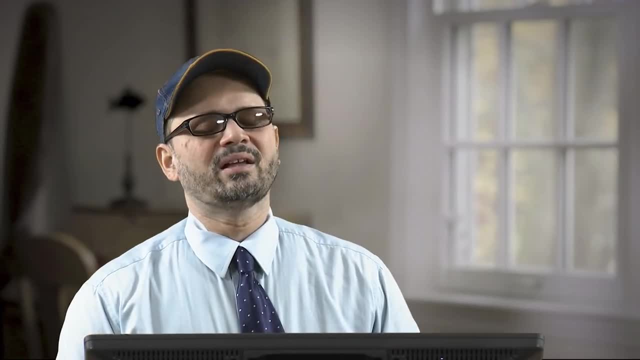 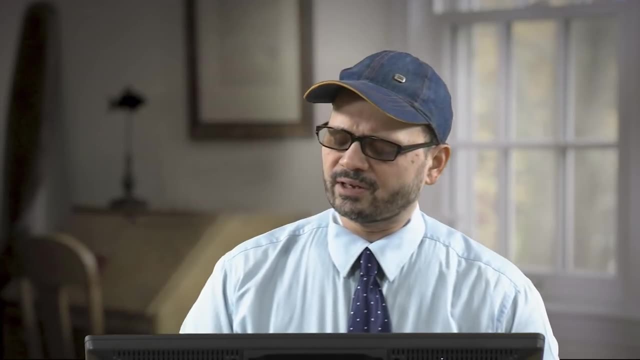 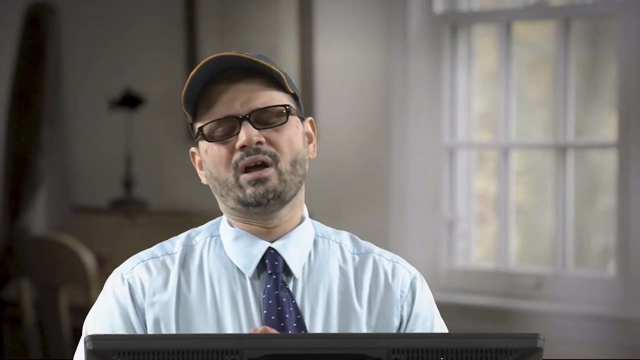 So basically bending and shearing process. normally they are applied in the case of the sheet metal forming processes and in the case of sheet metal forming processes, typically you go for such process: like we are punching, we are blanking, then bending of the sheets. 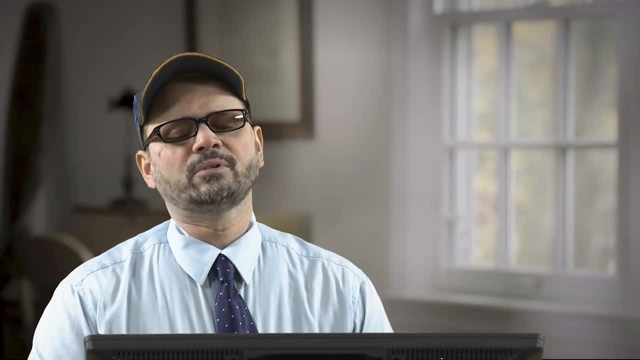 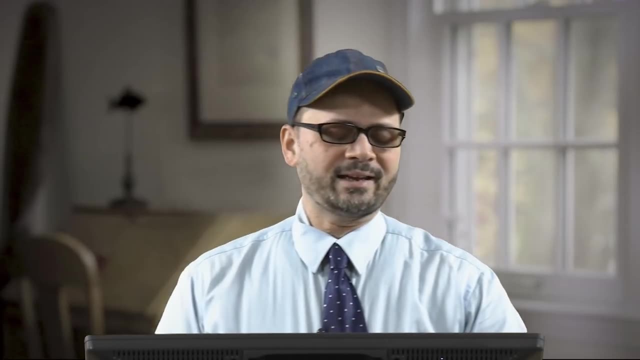 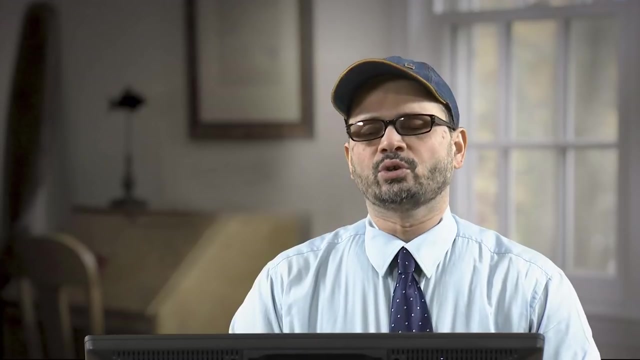 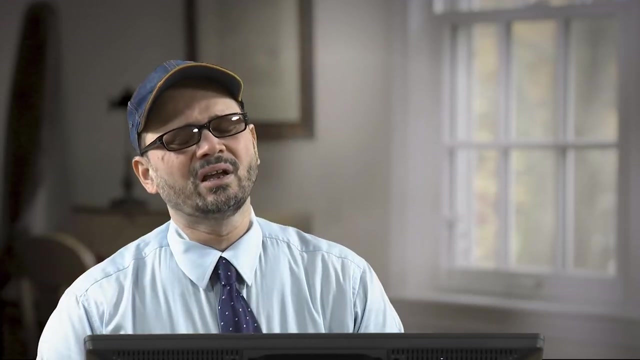 and all that. So there, these processes are basically utilized more and more. So then another classification is based on: you know what kind of operation you are doing. So what happens? that sometimes you are reducing the larger dimension, So smaller dimension, not the final dimension. you are achieving, final shape, you are achieving 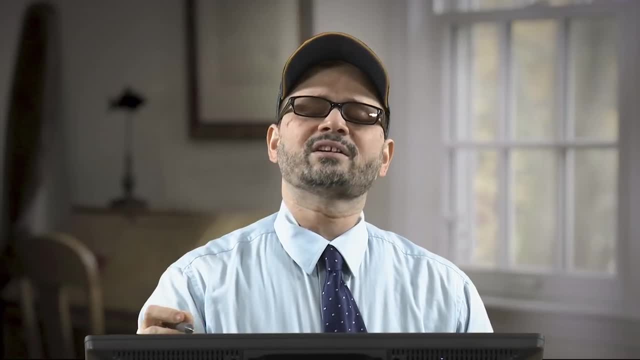 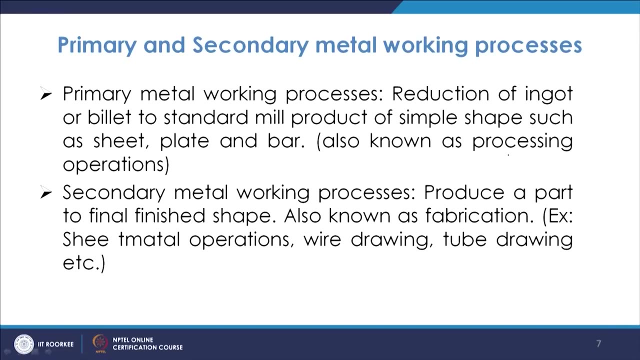 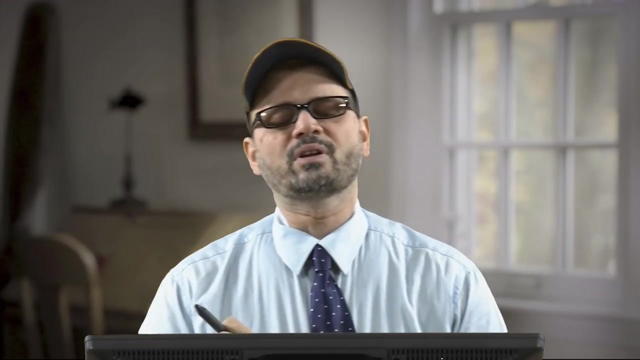 So when you are reducing the larger dimensional product like ingot or billet to standard mill product of simple shape such as sheet plate and bar. so that is basically the primary metal working processes. So you just like you do the rolling or the forging, or so intermediate one rolling basically. 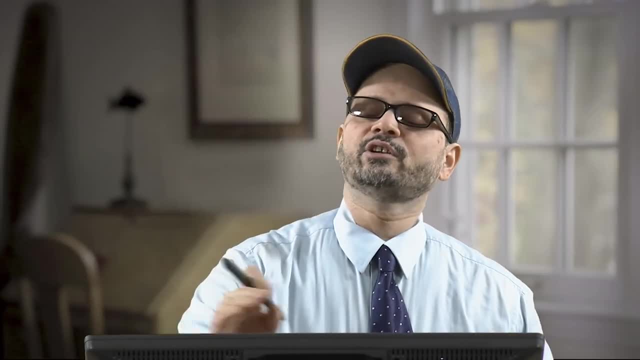 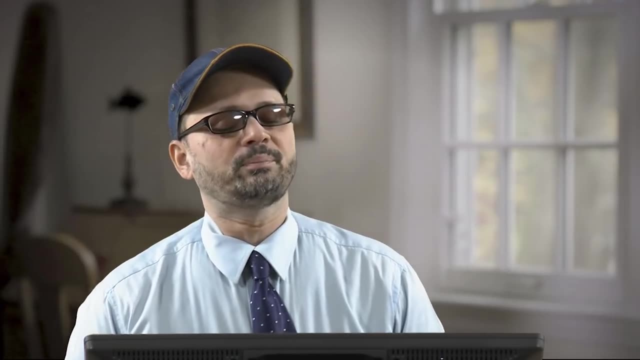 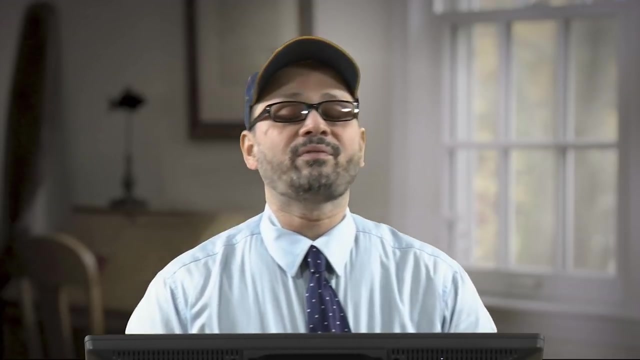 So those processes- So those processes are where you are basically reducing the larger dimension of the product to the smaller dimension- simple shapes- then that is your primary metal working process and then when you are going for the final finished product, So they are known as secondary metal working processes. 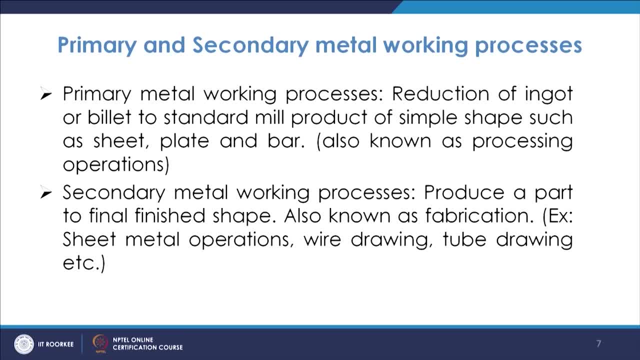 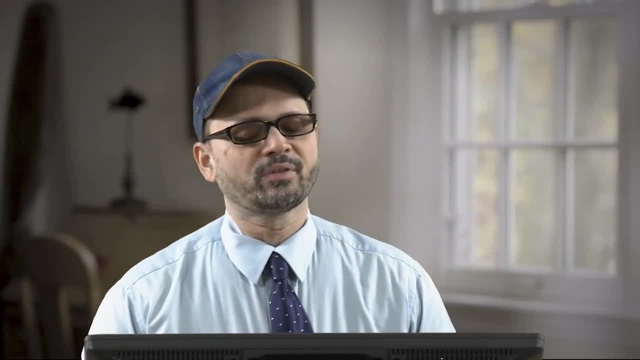 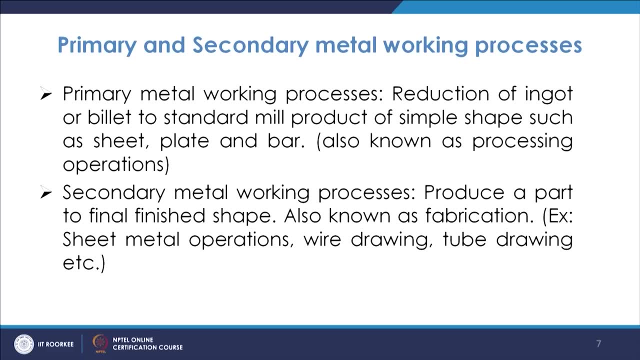 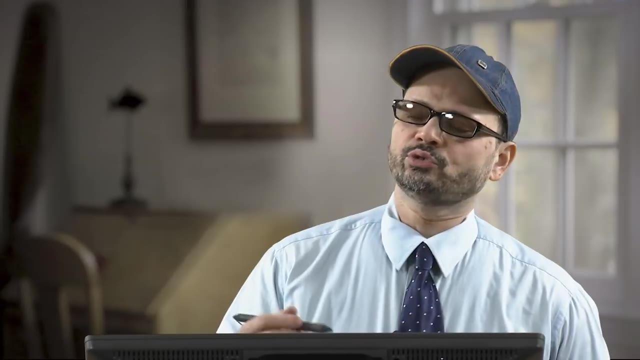 So in this case, what you do is you have to finally get the final shape. So the finishing is there, like the sheet metal operations, wire drawing, tube drawing, all these are the one which are the example of such processes. So in such case, you see that finally you get the final shape and the example is like: 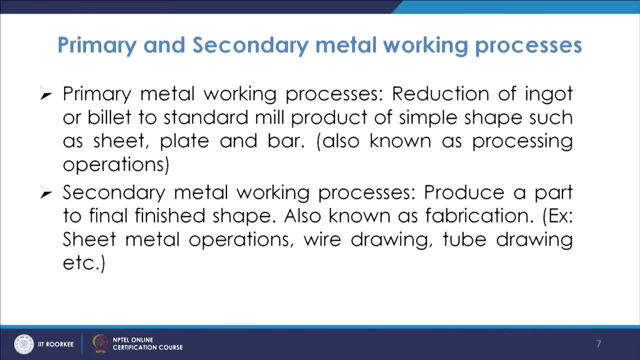 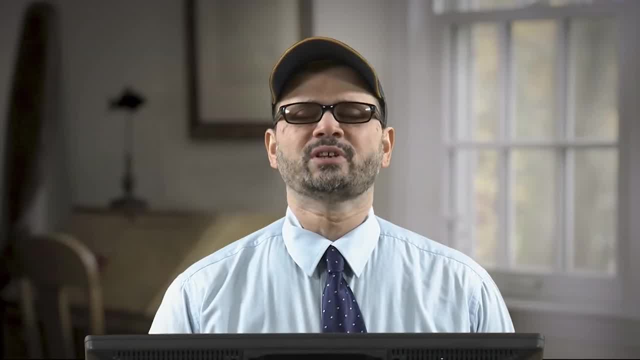 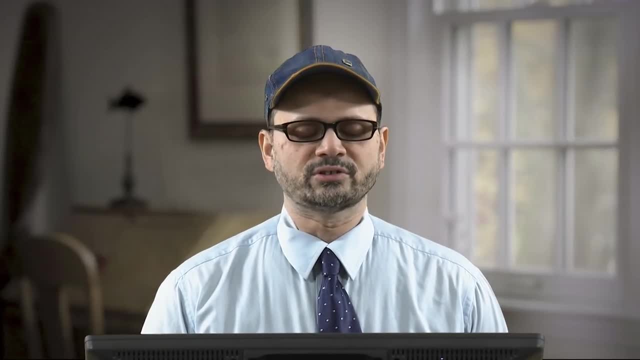 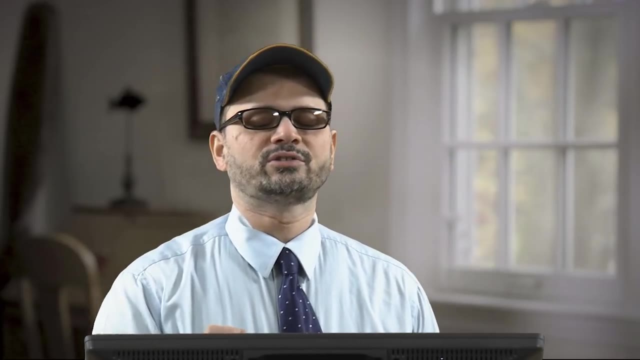 wire, drawing, tube drawing, etcetera. So these are primary metal working processes where you reduce the ingot or billet to simple shapes. they are known as processing operations and this is known as the fabrication operations. So normally it will be done on the larger size products- larger size, you know. sample. 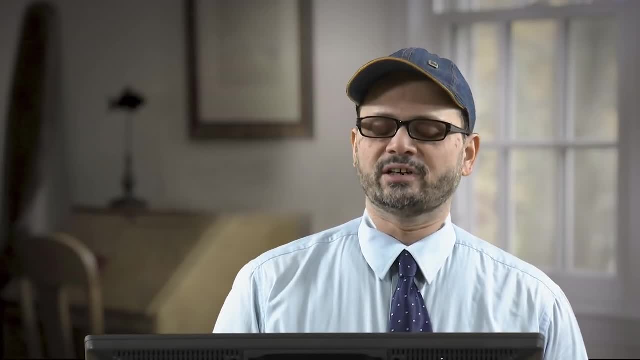 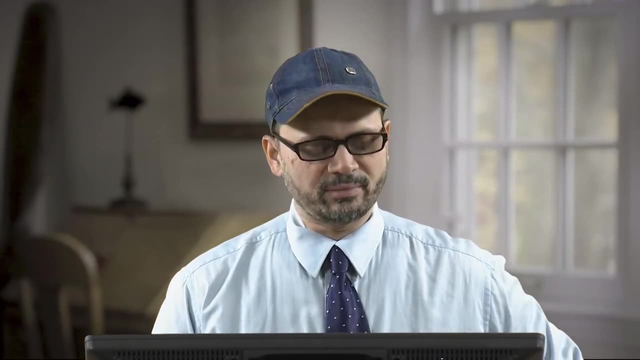 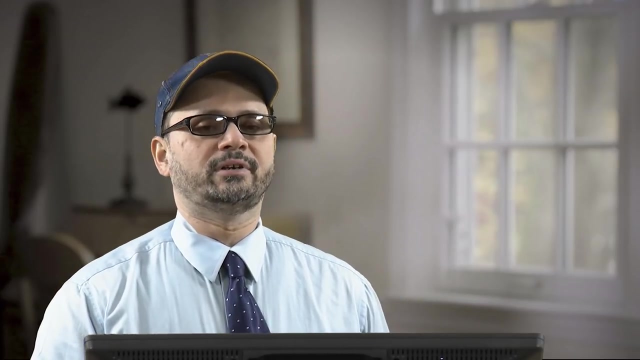 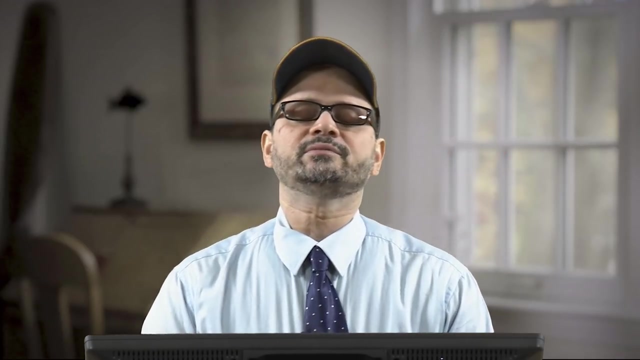 like billets or the ingots, and here it will be done on the sheet metals. so that is known as fabrication. So fabrication operations, that is secondary metal working operation. then we already discussed that you have the classification, also based on the temperature of deformation and the 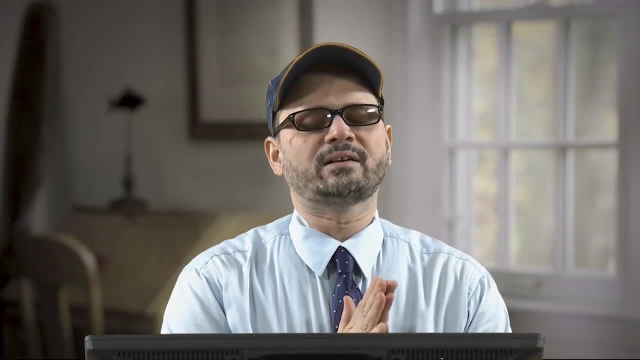 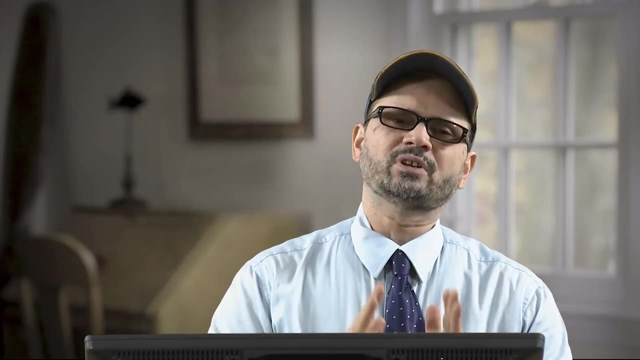 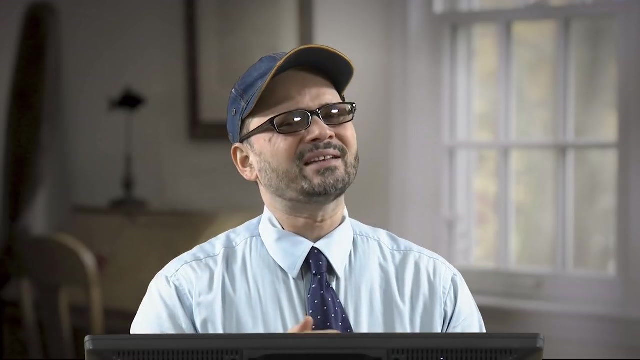 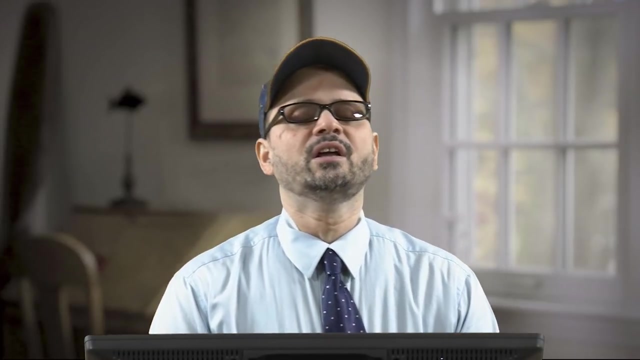 temperature. on the basis of temperature, it is defined as either hot working or cold working. So, as we know that there are two main purpose purpose of doing the deformation, one is the reduction in dimension, as well as the improvement in mechanical properties and, many a times, the improvement in the strength. 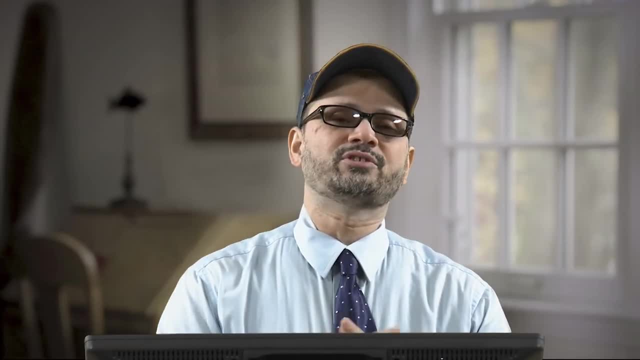 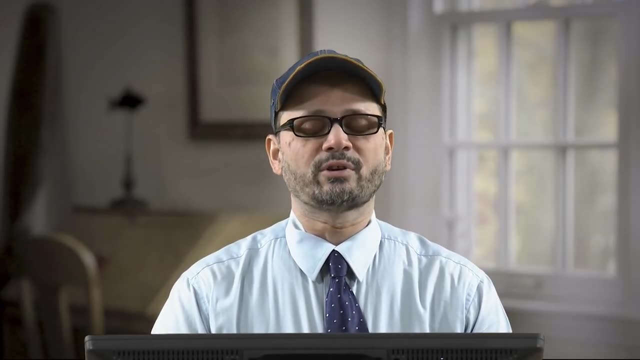 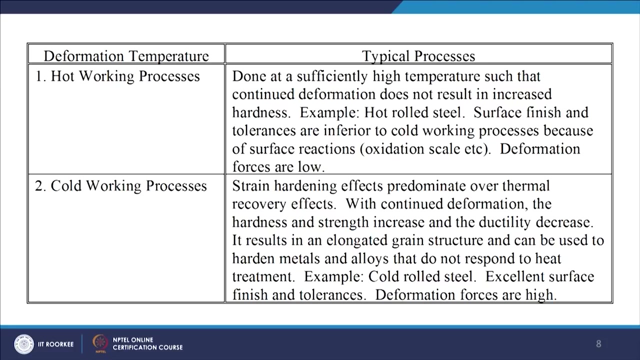 So the deformation, when we do at higher temperature for getting larger deformation, then it is known as hot working or hot forming processes, and it is done at sufficiently high temperature. So in that the deformation will be more, but the hardness will not be more hardness. 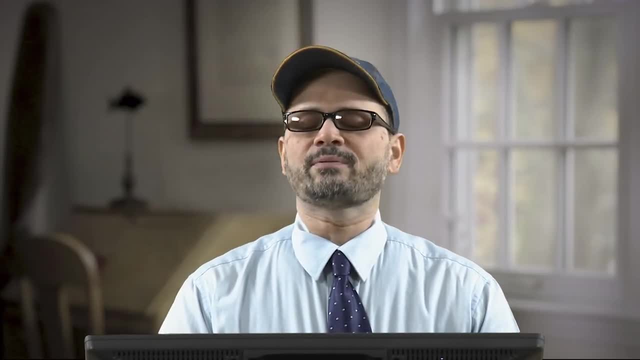 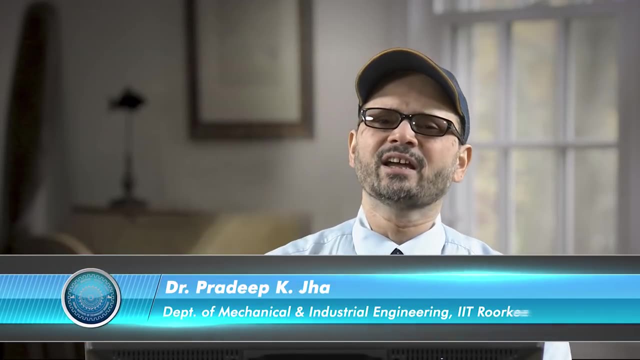 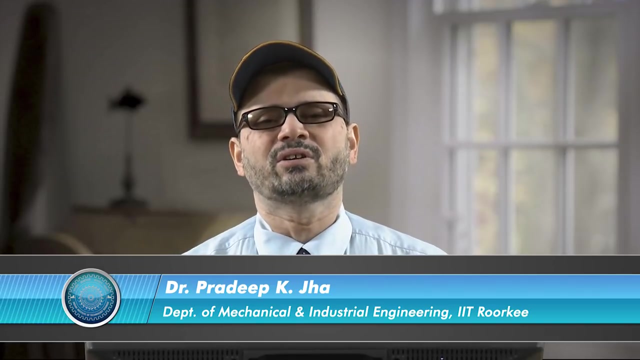 will not be increased. So also the surface finish and the tolerances are inferior. So we have discussed that in the case of hot working, since we are dealing with high temperature, So there will be at high temperature there are chances of the scale formation and you. 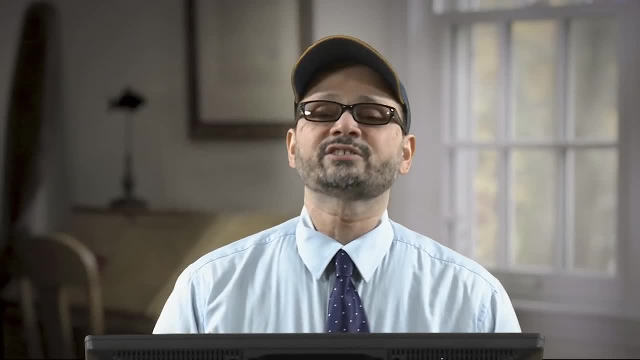 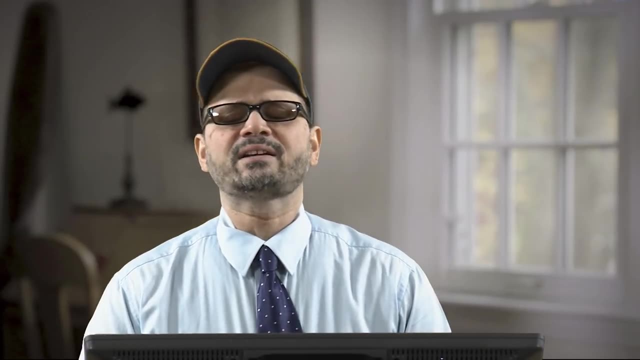 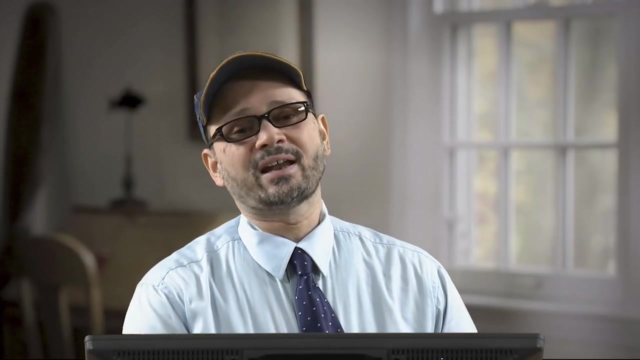 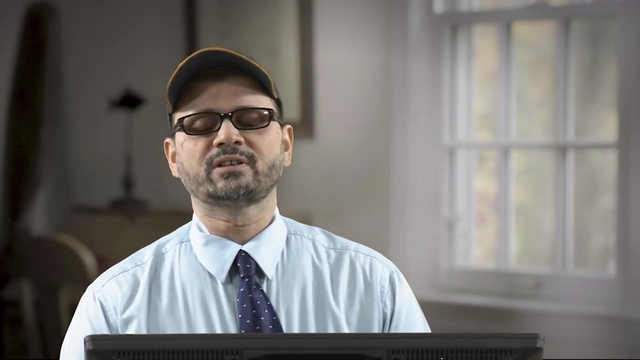 cannot control the surface finish, Surface finish and also the dimension to a very precise value. So basically, in that your surface finish and tolerances are inferior as compared to cold working because in cold working it is done at lower temperature, So they are the finishes better. also, there are surface reactions like oxidations scale. 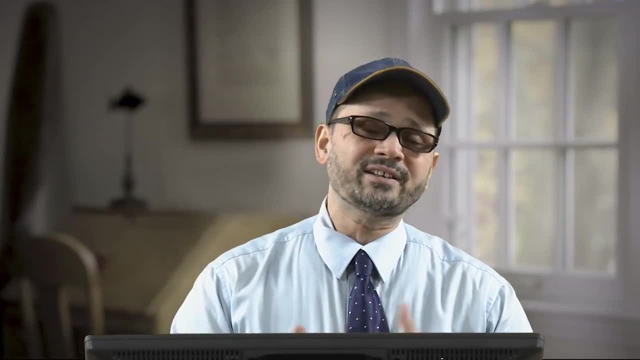 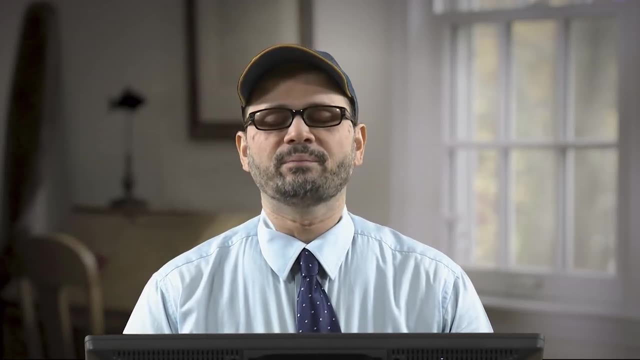 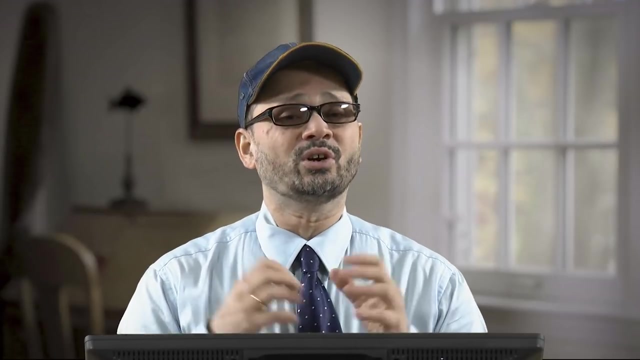 and all that. So that is that another advantage of the hot working is that the deformation forces are low. So in such cases, when you increase the temperature the material becomes, it is strength becomes less, So the force which is required to deform the work piece is low. 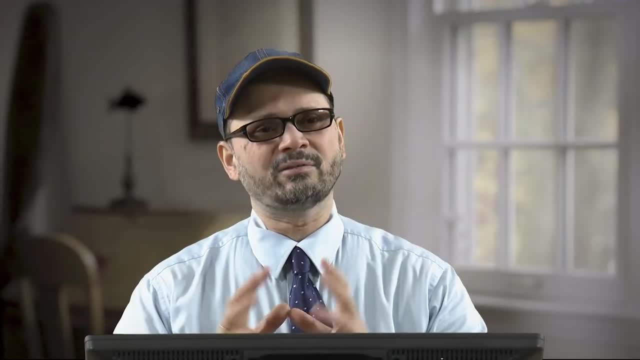 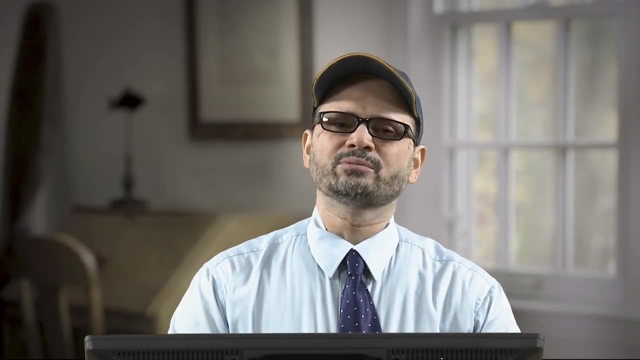 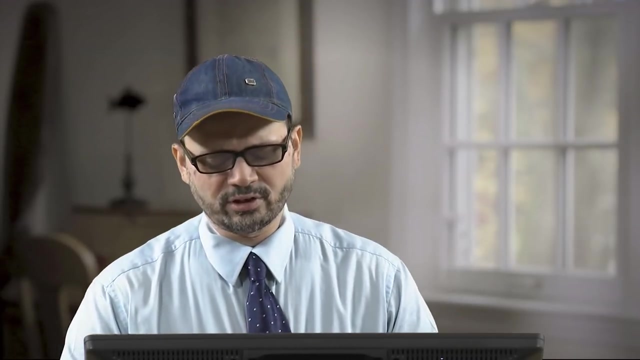 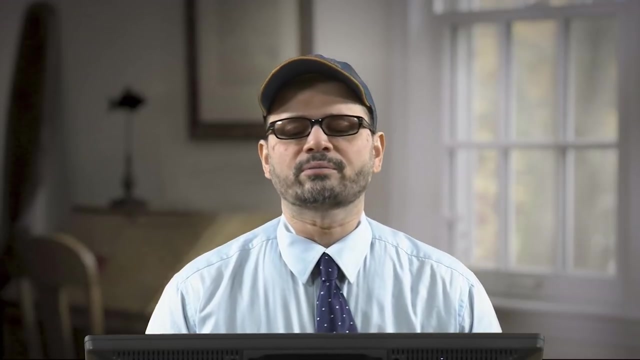 So you can go for larger degree of deformation, whereas when you go for the cold working at, as the temperature comes down the strength becomes higher, So in that case the requirement of the load becomes larger, So that there is a limitation up to what degree of cold work you can go for. 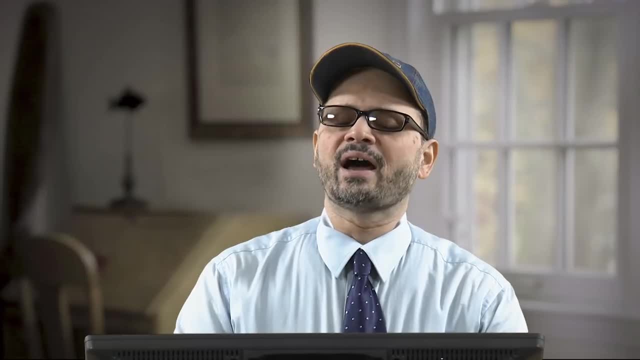 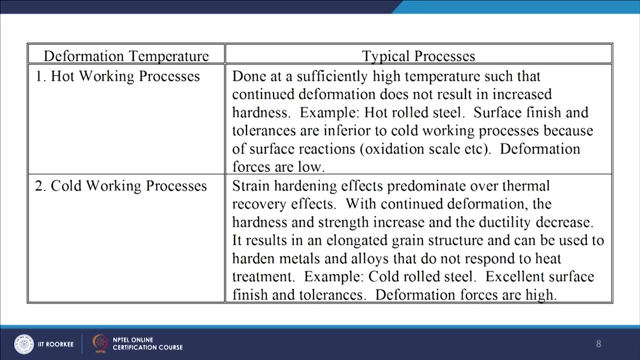 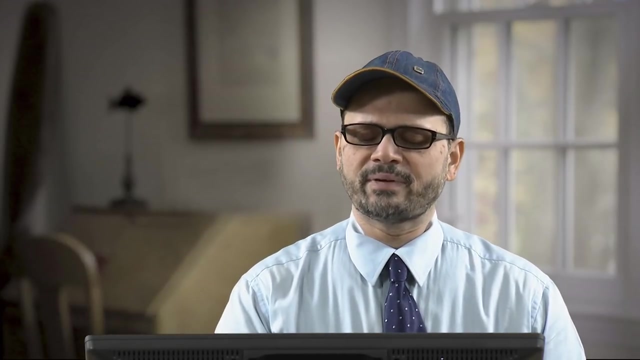 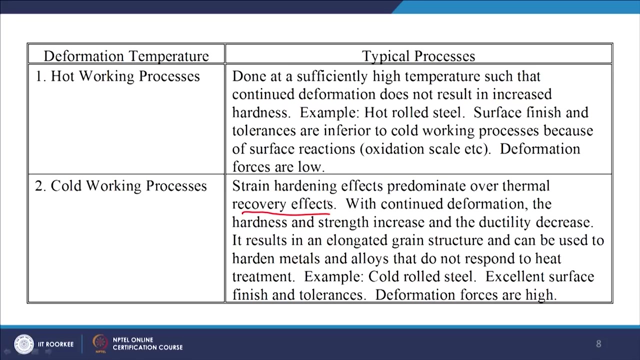 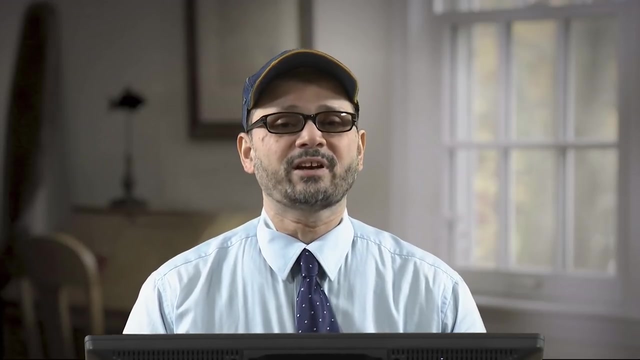 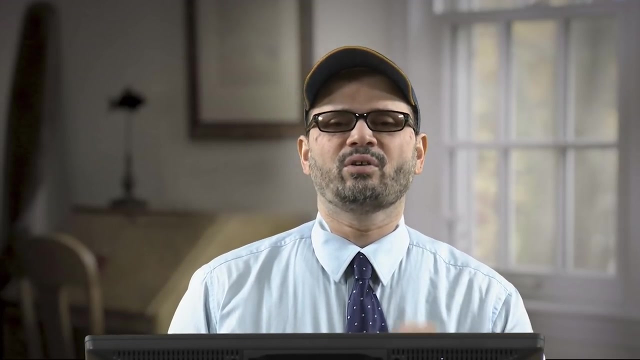 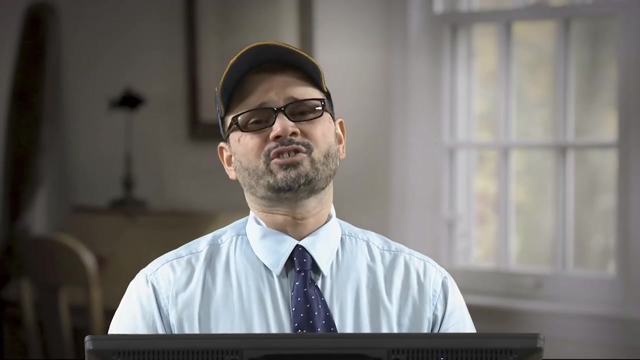 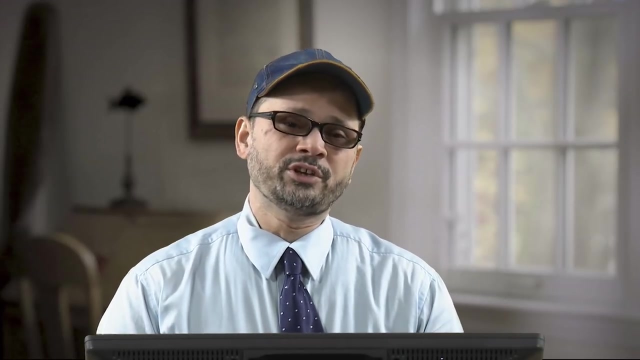 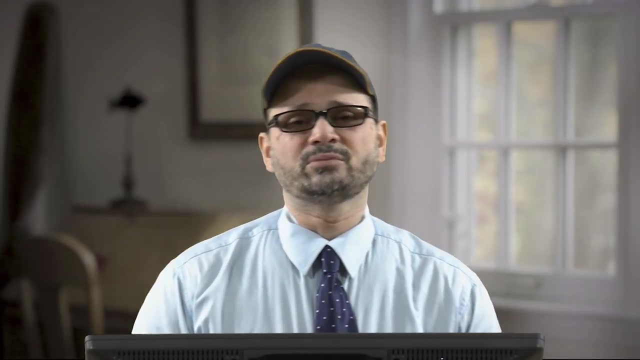 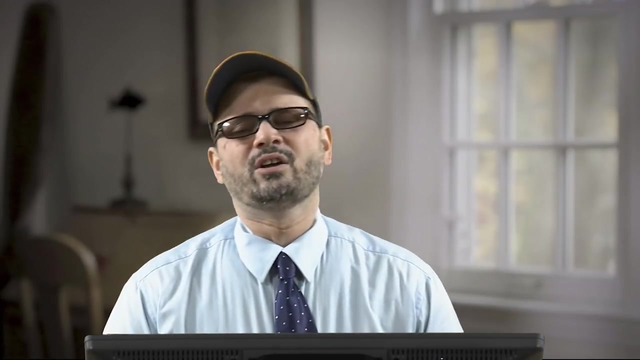 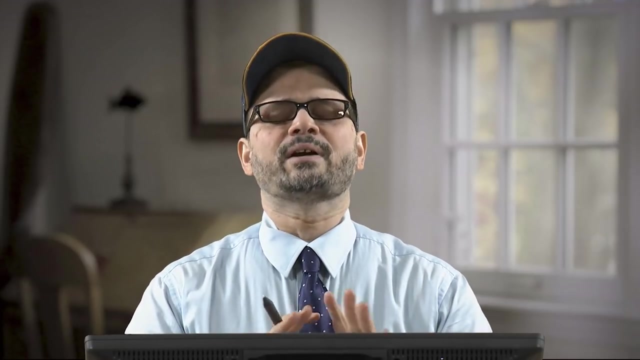 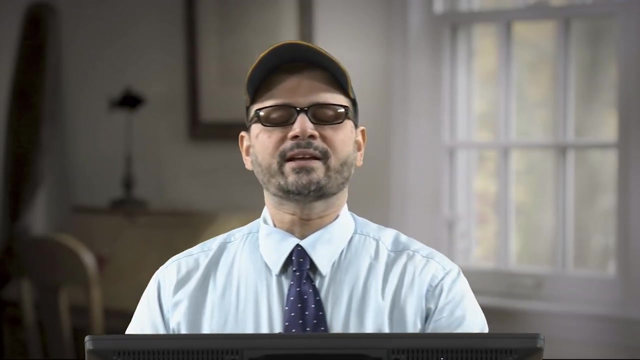 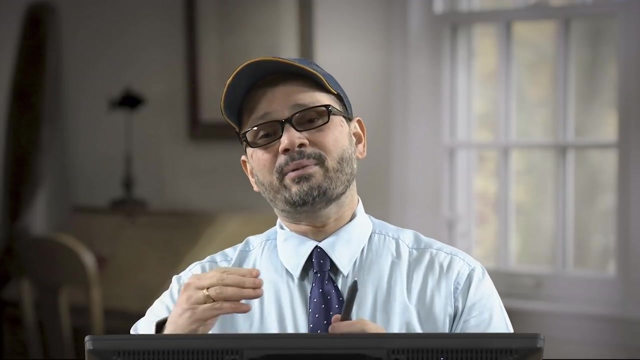 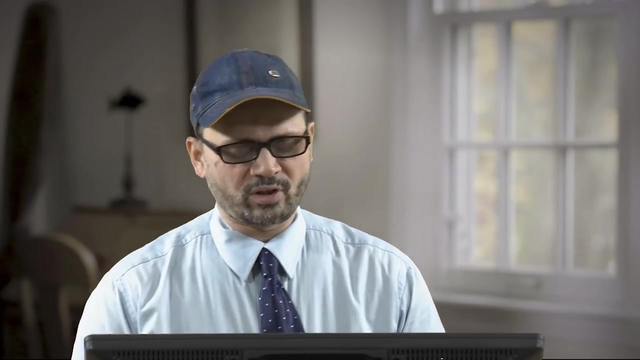 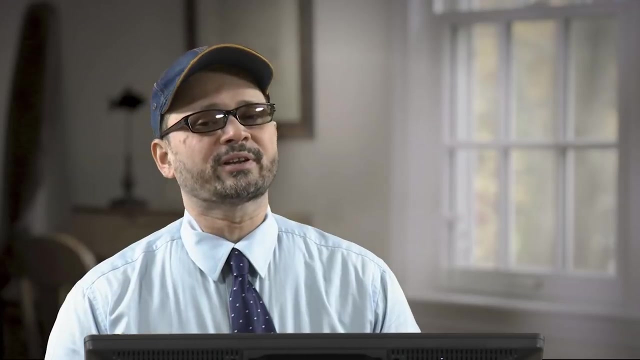 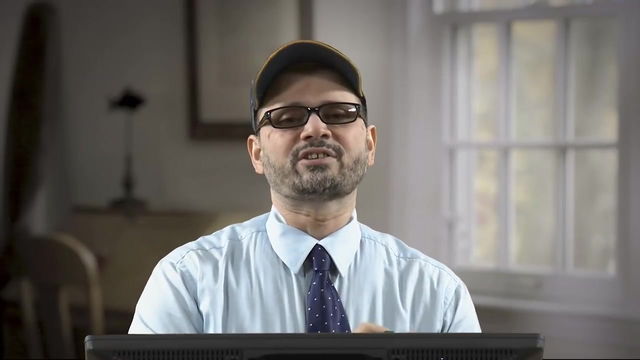 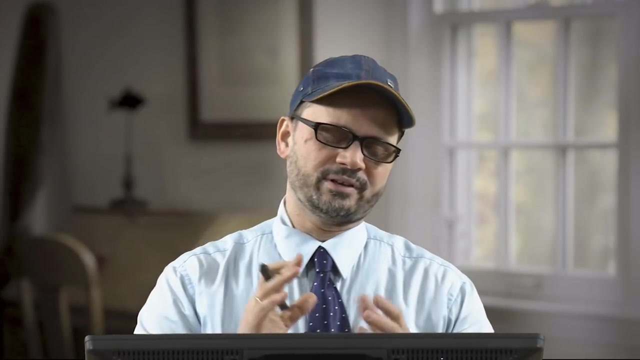 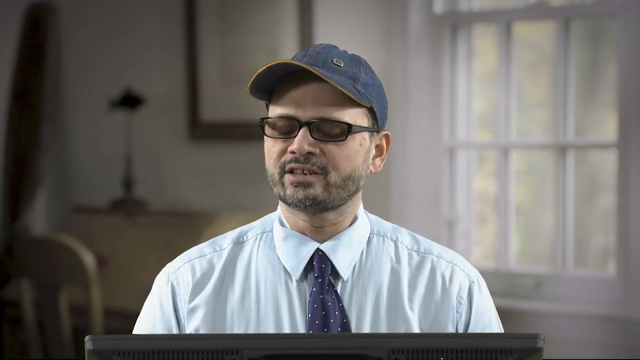 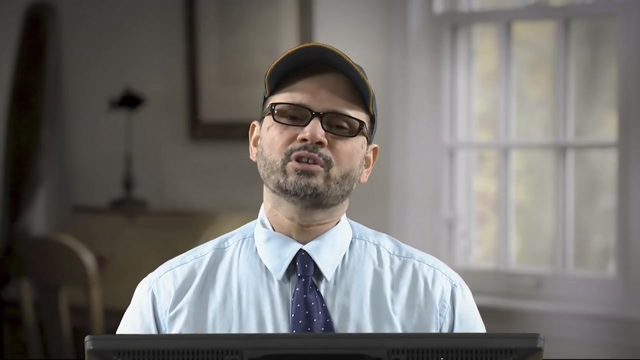 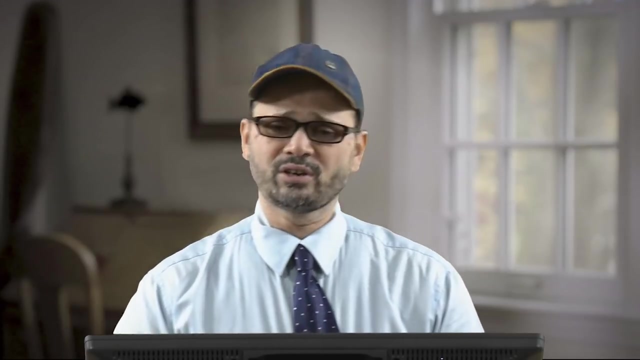 So in the case of cold working process, the strain hardening effects predominate over thermal recovery effects. So, as we discussed that, the main difference between the hot working and the cold working is, that is, this recovery effect. So in the case of cold working, the heat treatment will, not the ductility, to certain extent the ductility will be decreasing, So it results in an elongated grain structure and can be used to harden metals and alloys that do not respond to heat treatment. So many a times those materials which do not respond to heat treatment you can go for. 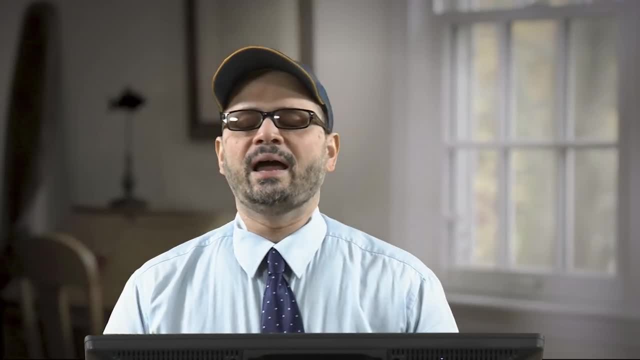 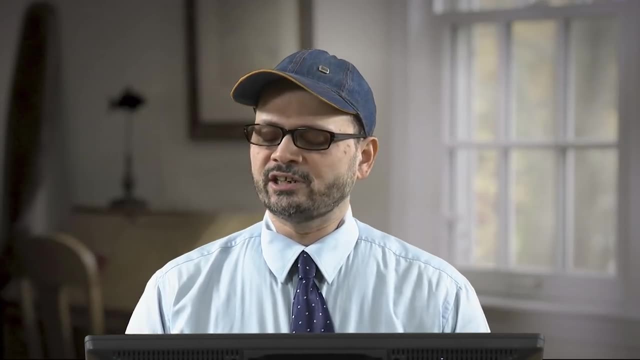 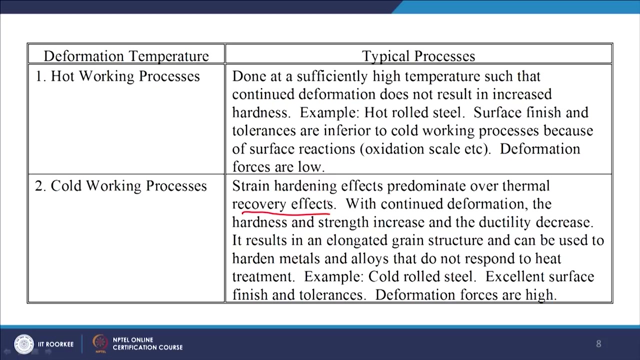 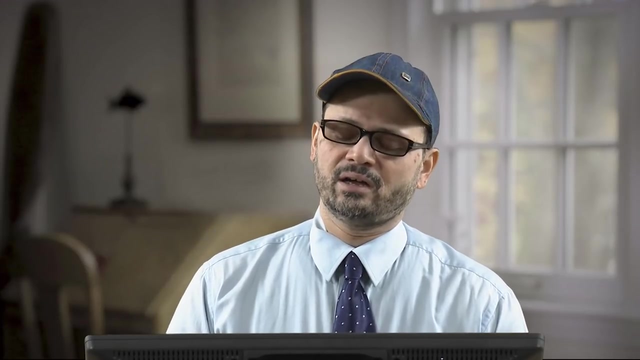 such treatment to such metals, such materials, and get their proper properties improved. example: cold rolled steels, So excellent surface finish and tolerances and deformation forces are high. So, as we discussed, that when we are dealing with the material at higher temperature, as well as low temperature. at lower temperature the yield strength is higher. So for deforming you require larger and larger forces, and as you go on cold working every time, So in the case of cold working the strength will be increased. So you require larger stress further to deform. So deformation force will go on increasing, you know, as we go continuously deforming the material. So there is a limit of the degree of deformation in the case of cold work because you need very, very high powered equipment. I mean, if you try to do the, you know, cold forming, cold working beyond certain degree. then the material may be broken. it may be, it may result into fracture, because the brittleness is induced in the material. So this is the basically difference between the hot working and the cold working. Now, that is basically depending upon the temperature, and this temperature is a recrystallization. Temperature, as we discussed, and this recrystallization temperature is normally 0.5 to 0.6 times the melting temperature of the material in Kelvin. So if you take about the iron or so, about 1000 degree or so in case of steel, low carbon. 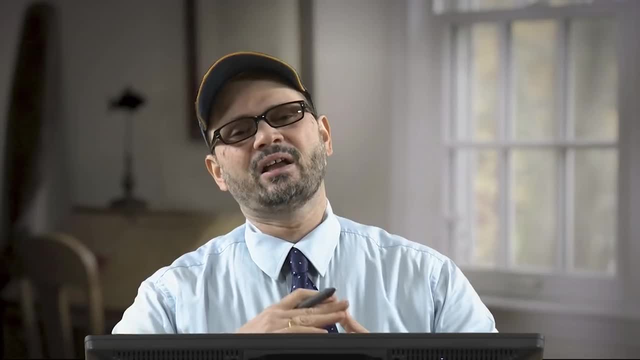 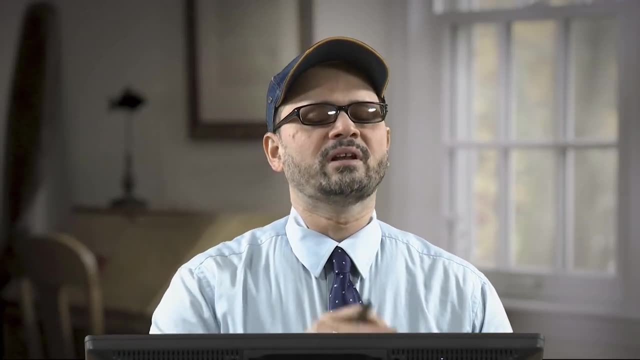 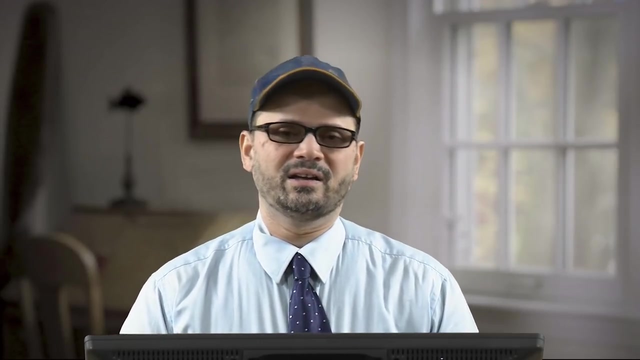 or medium carbon steel in case. So if it is deformed above that, then it is the hot forming and below that it is a low. which is low? I mean hot working, or it is below that, it is cold working. Now the thing is that many, for many metals, the, if you look at the recrystallization temperature, 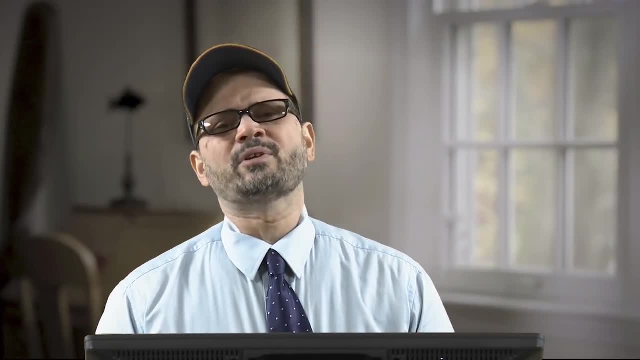 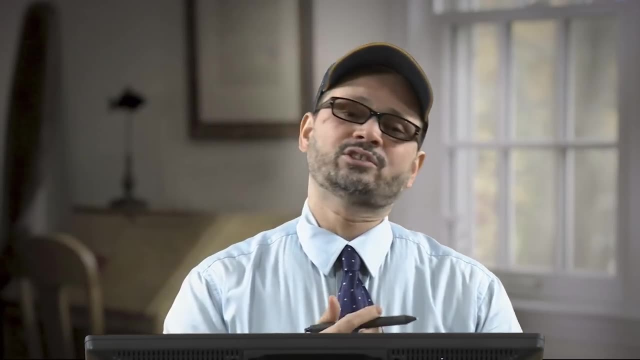 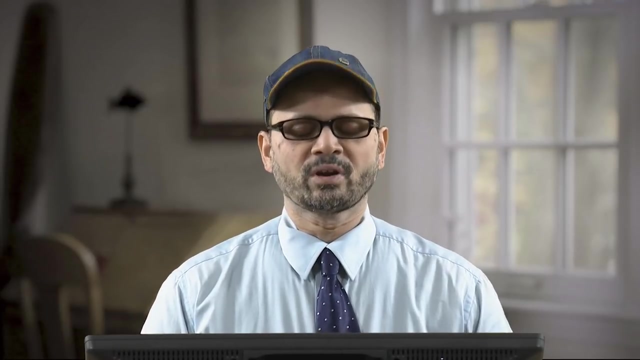 it is not very high value. So even the room temperature may be the hot working temperature. So you have to keep in mind that. so in those cases that is a cold working itself or a hot working itself, So it depends upon the room temperature, whereas in the case of iron you have to go. 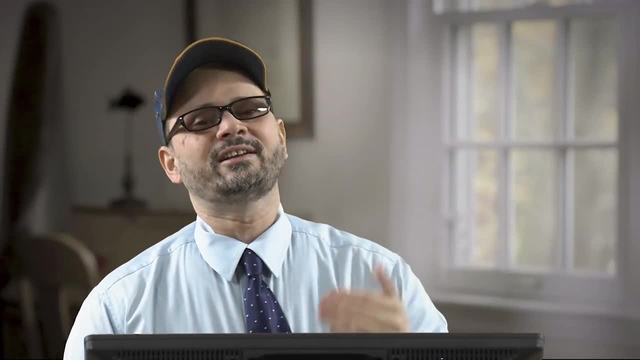 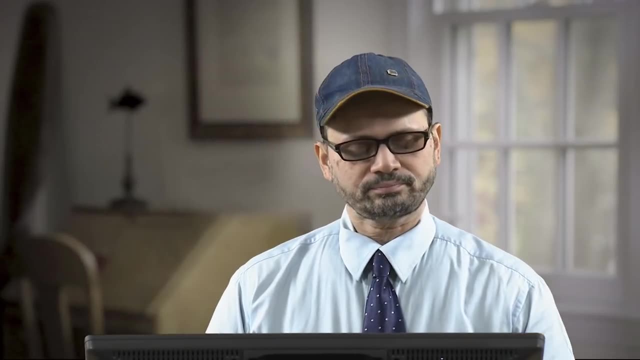 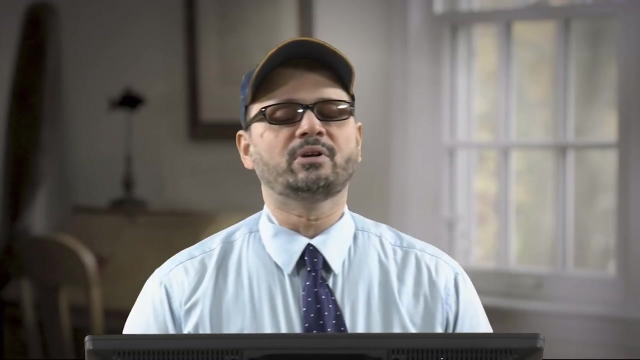 for very high temperature and even if you go at 600 degree centigrade, it is a type of cold working, So that it depends upon the materials properties. Now we need to know about the deformation processing system. So what is the deformation processing system? 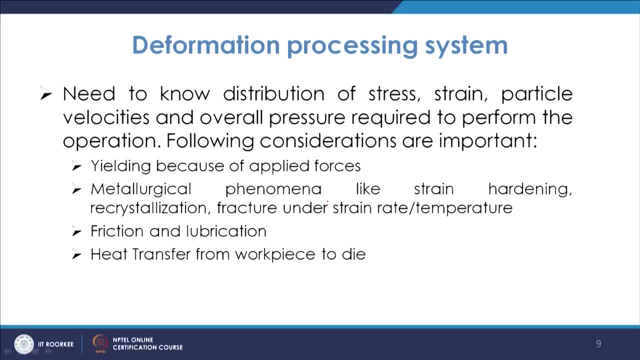 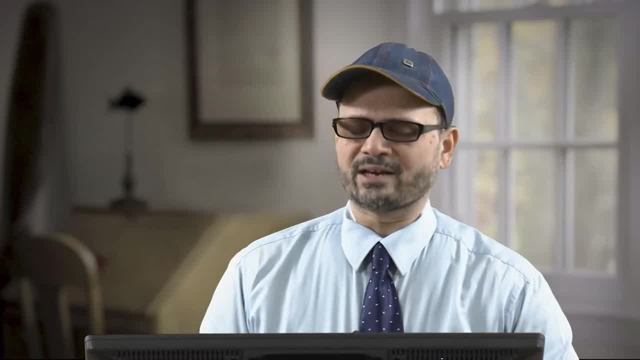 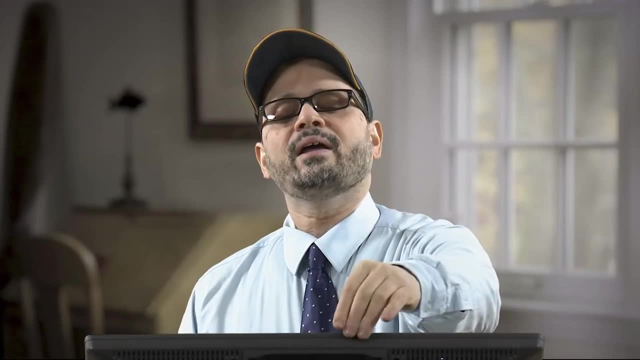 So when we talk about the deformation processing system, I mean it is a domain where your you have to pinpoint that what you have to study Now, when we talk about any deformation process, what is typically there in a typical deformation process? 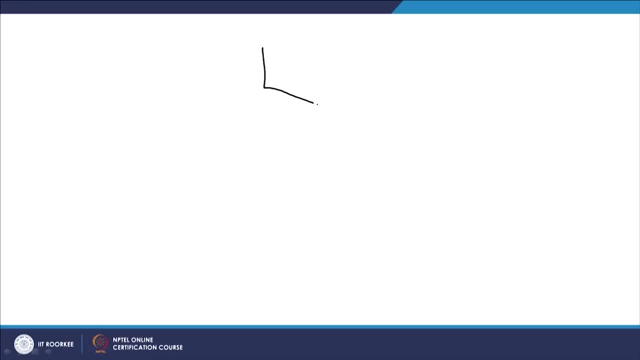 So what happens that you have suppose, such is the material, such is the, this is the die, This is the top die and this is your bottom die, and you are allowing some material to suppose go there and then it will go through it. ok, 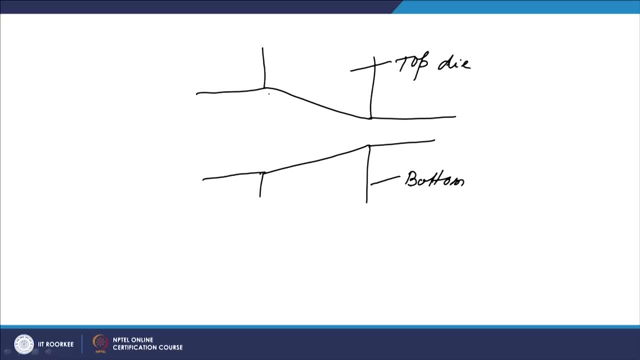 So the thing is that what happens? that this is the die and this is work surface, work piece. So, basically, this zone is the lubrication zone. lubrication zone is developed here and similarly, you will have a lubrication working here And here itself. similarly, you have you know if you look at this zone, this is this zone. 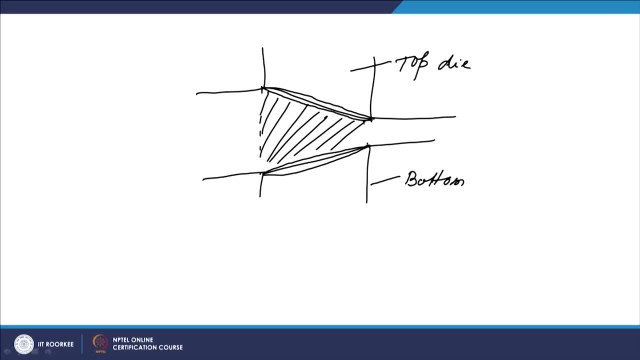 is basically the deformation zone, So this zone is known as deformation zone. So this is the zone known as the deformation zone and this is your top die. similarly, this is your top die and from here is the material is pushed and it comes like this: 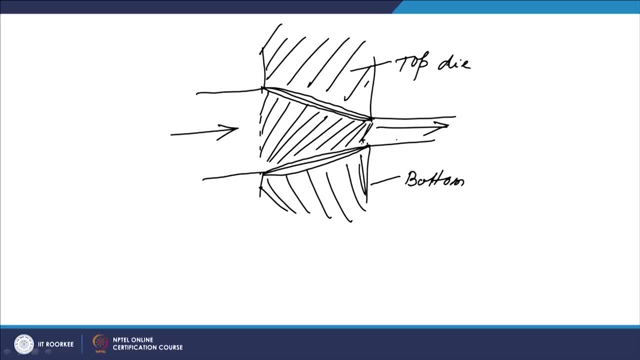 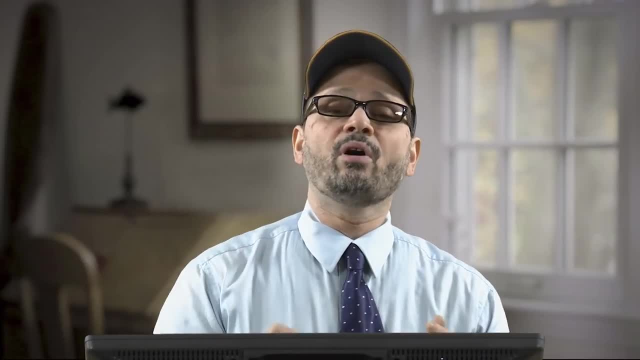 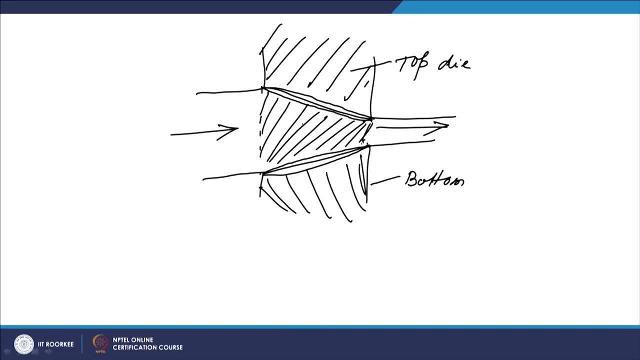 Now the thing is that you need to concentrate, To concentrate on this zone, and you want to find what is the stress, strain value, velocity, what is the pressure required to deform, all that you need to know. Now the thing is that when the, the material which you put, is heated here, 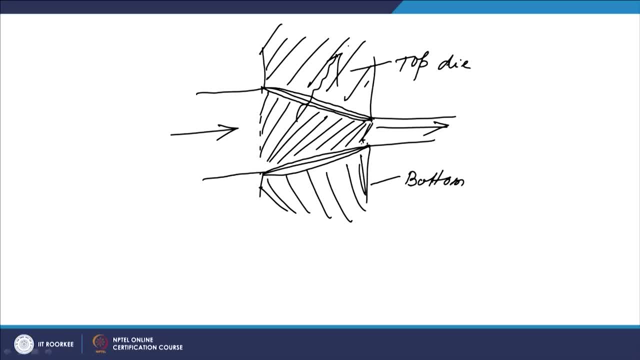 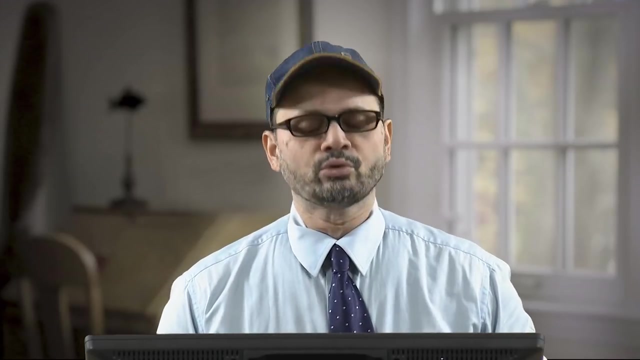 So what it will do, it will be releasing the work heat to this side. So, basically, there are many things happening in this zone and this zone is known as deformation zone. So in this, what we do in the case of deformation processing system, we need to know the distribution. 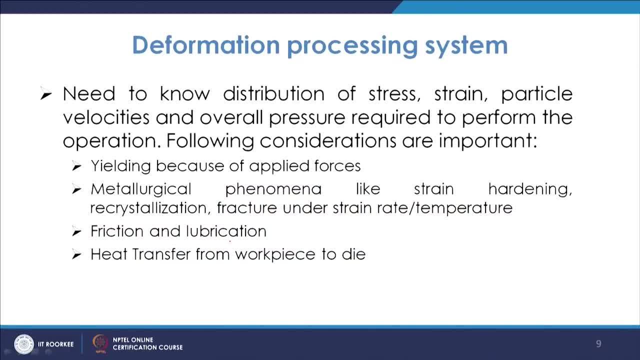 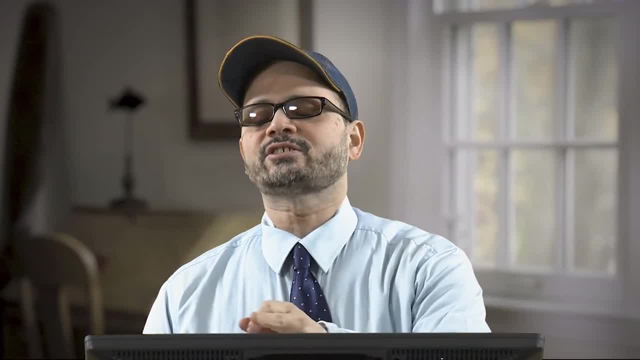 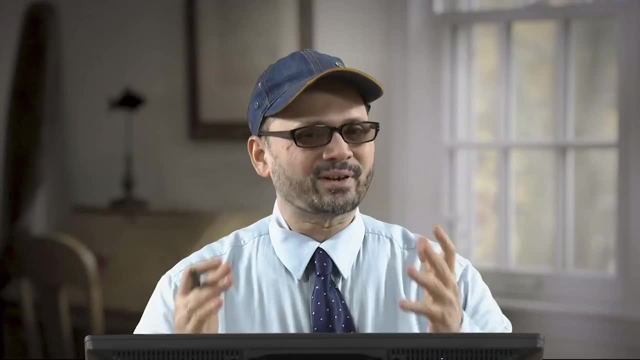 of stress strain, particle velocities and overall pressure required to perform the operations. So that is what we need: we need to find the stress strain velocity and also the what is the pressure required to perform the operations. So based on that, you can design the equipment so that you will be doing the successful forming. 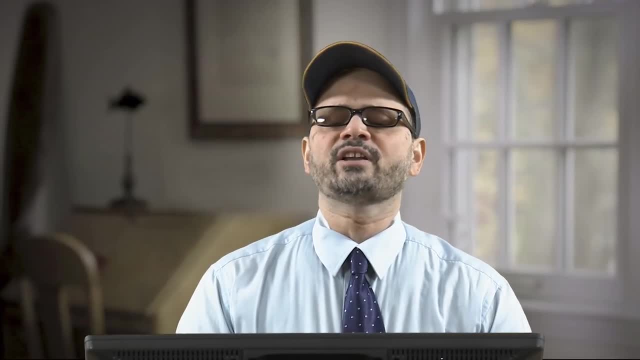 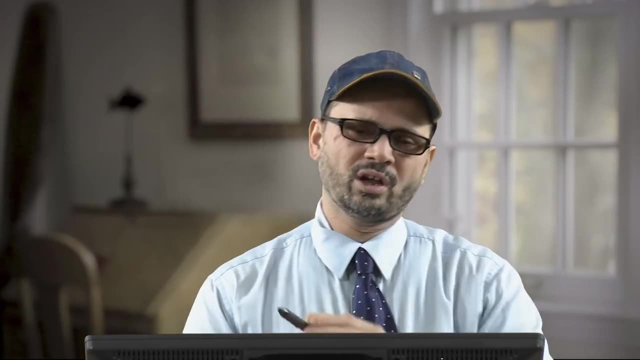 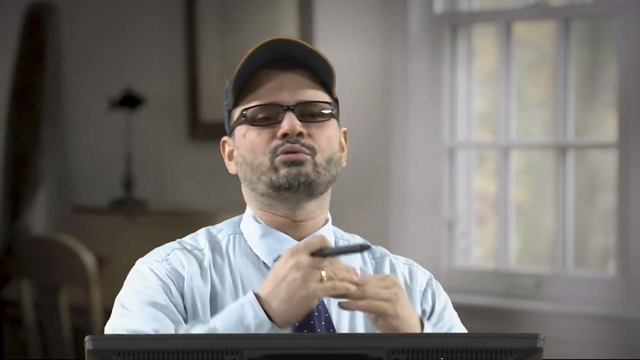 operation. Now, for that there are many things, many considerations which are important. there will be yielding because of the applied forces. So in the deformation zone, when you are applying the forces, then the material yields. when the stress value will reach beyond or equal to the yield point value, then the material 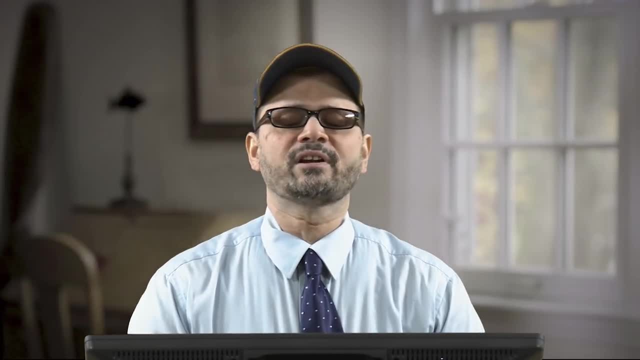 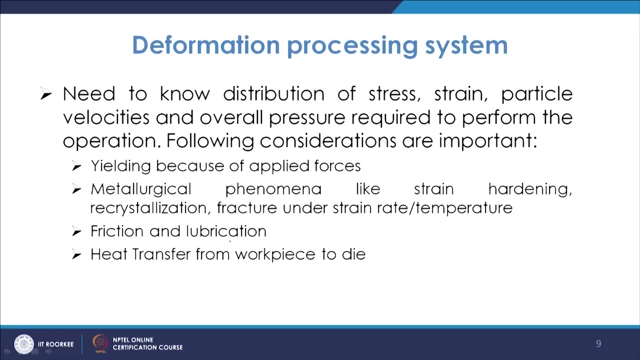 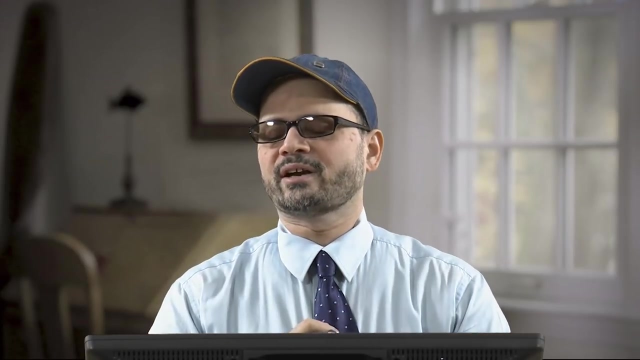 will yield. Similarly, there are many metallurgical phenomena, like you have, strain hardening, recrystallization fracture under strain rate and temperature. So you have, there are many parameters which are to be taken into account, like, depending upon the temperature conditions you may have, the strain hardening effects you may have. 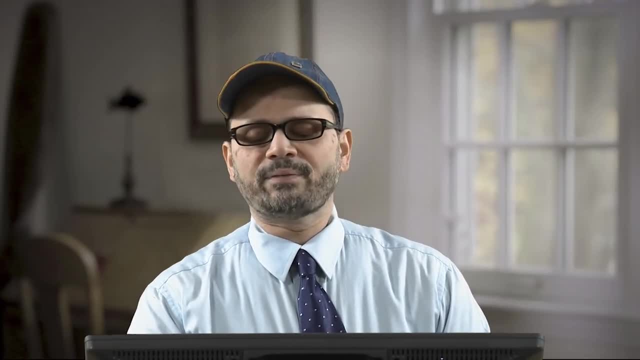 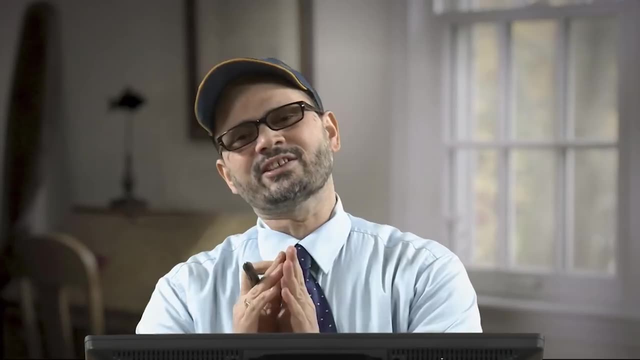 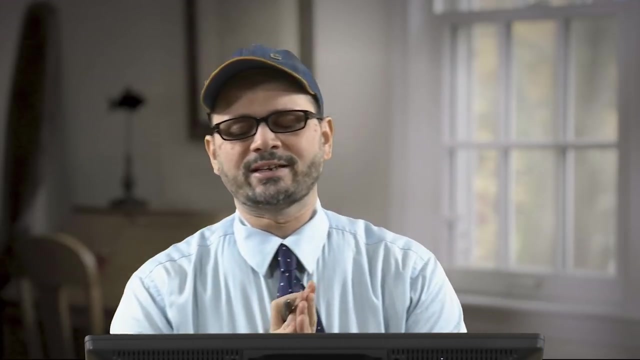 the recrystallization effects. Also, the fracture will be there under the strain and strain rate and temperature. So there are strain, is there strain rate, So there, strain rate is there. and temperature. These parameters affect basically the fracture behavior in one sense. 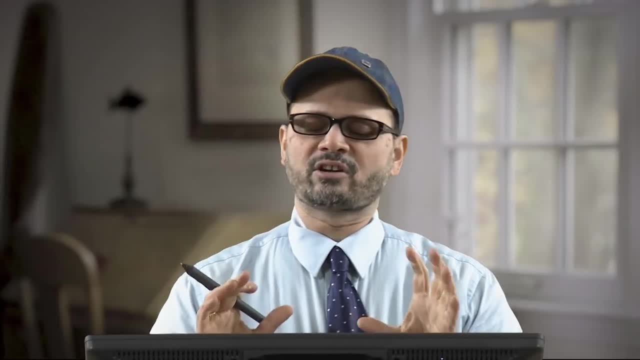 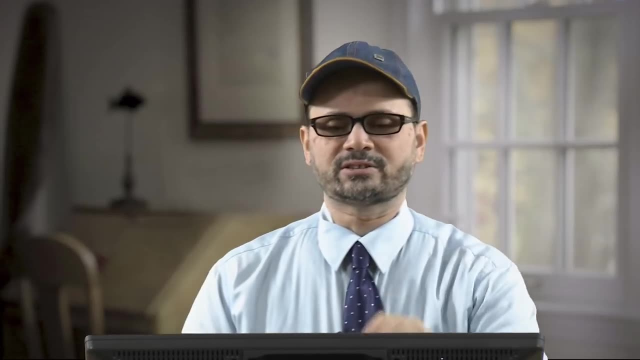 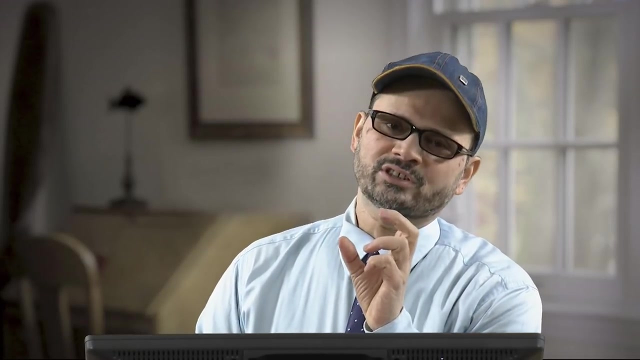 And so you need to have a consideration of all these effects. you have friction and lubrication going on. So, as we discussed that at this place, when it enters into it there will be friction forces and then you are applying the lubrication system here. 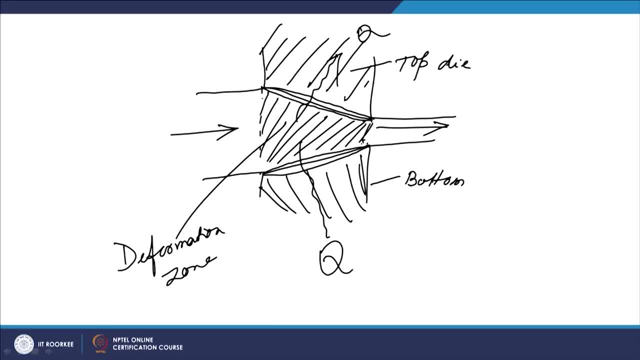 So there will be friction forces and then you are applying the lubrication system here, So these also need to be tackled. when we talk about the deformation processing system, We need to see that how much friction is generated. Friction forces are required so that the material goes into this and then the slowly it will. 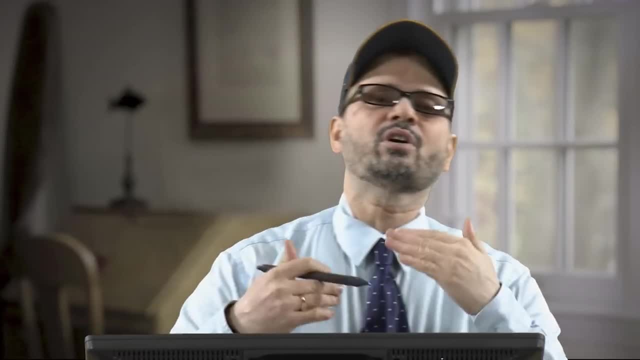 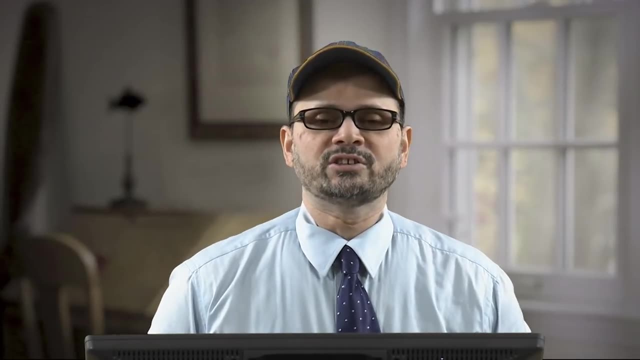 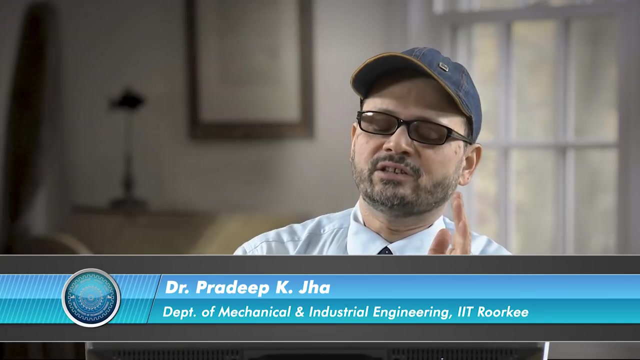 come at and then it comes out here. So, basically, when we talk about the different type of processes, we will see that how these friction forces play their role in pushing the system into in between the rolls or in between the dies, And then how the friction is, you know, generated what will be the frictional forces amount? because 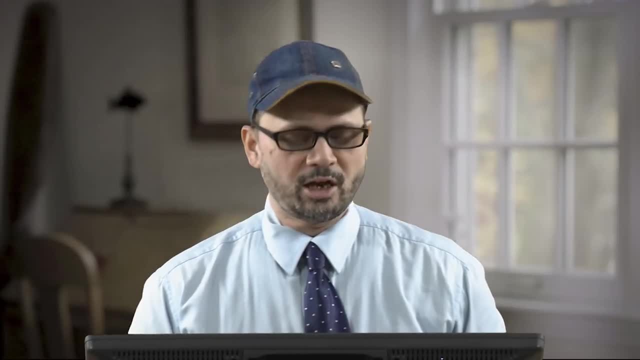 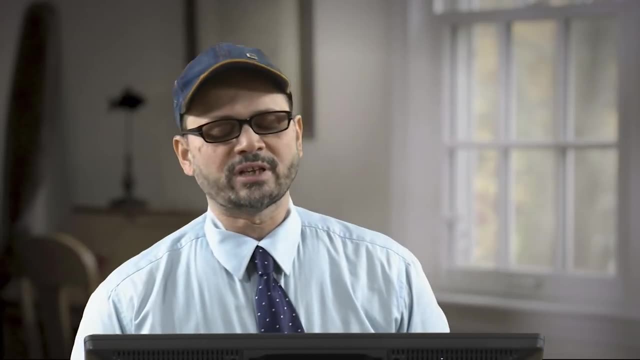 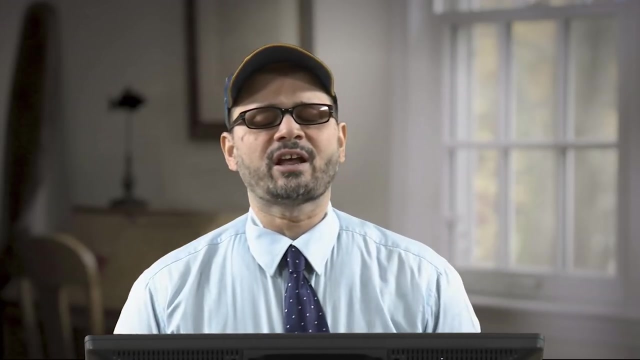 depending upon the reaction amount, you can have the frictional amount. what should be the maximum friction or minimum friction which is required? So that is another consideration which has to be kept in mind in such cases. Then there will be heat transfer from the work piece to the die. 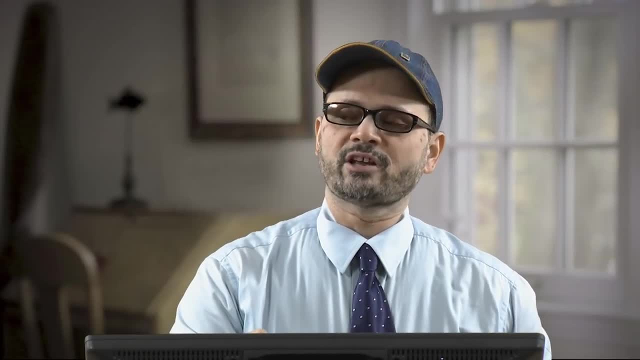 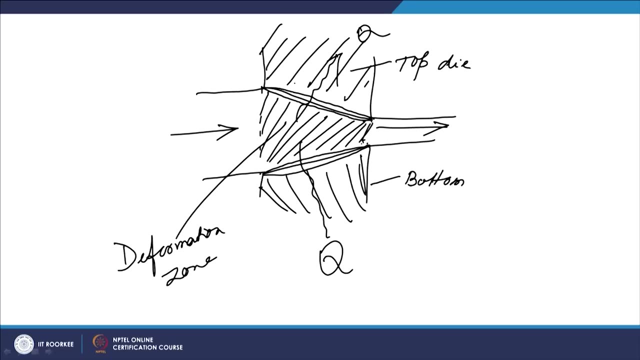 So that is what we have. We have seen that your heat will be transferred from this side and it will going into the die. So from the work piece it will go, because it is in intimate contact with this. so heat will be transferred. 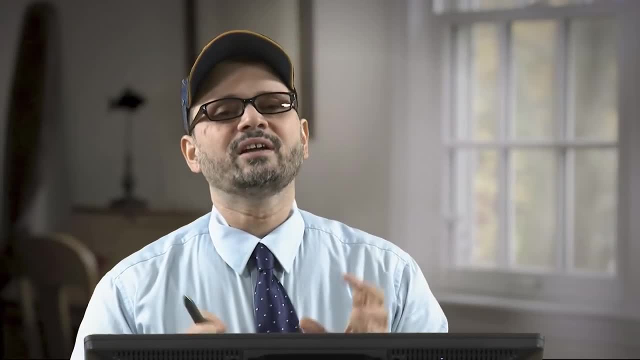 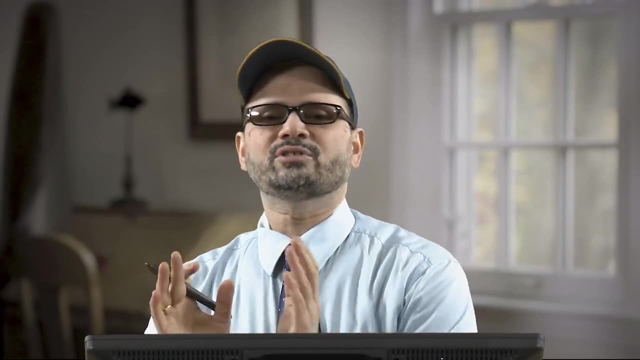 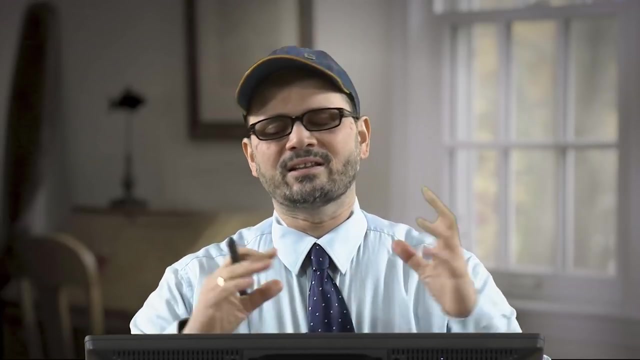 So all these considerations are required to study about the deformation processing system. So as we discuss about the different processes, we will see that how the deformation goes, which zone you have to confine yourself. to study about the processes, Ok. And to find further the value of pressure or stresses required to deform velocities.